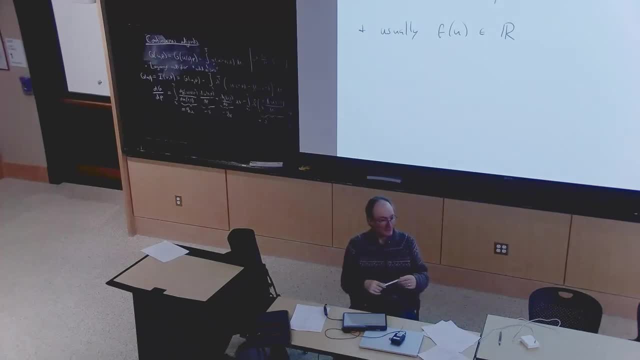 vectors. they're even matrices. You can even think of functions as as a vector, because you can take two functions, you can add them, You can take two and get another function. You can take two functions and multiply them. a function and multiply it by two and get. 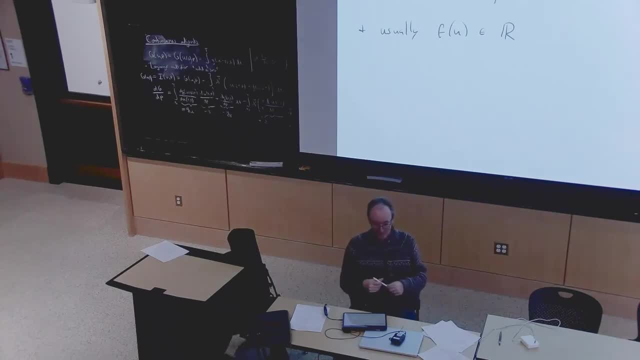 another function And so a lot of the things you can do- linear algebra for column vectors- you can do for functions. right, You can talk about linear operators on functions, like a derivative is a linear operator in function. You can talk about orthogonal functions and 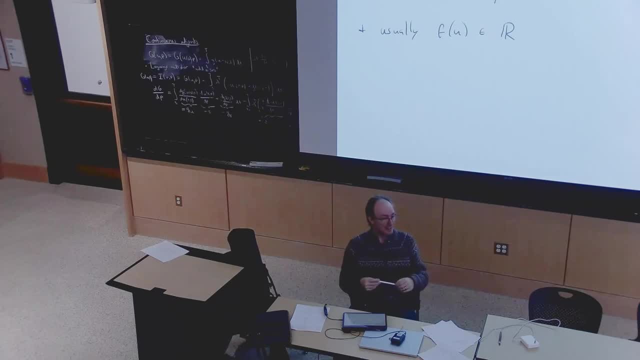 dot products of functions and Gram Schmidt on functions and Eigen functions. if you do quantum mechanics, you do lots of things with Eigen functions, right? So you know it's the same same, all the the same kinds of concepts. You have to be a little bit careful. 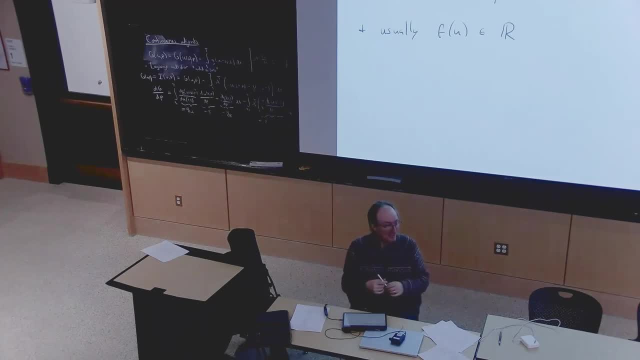 I think that's pretty useful. I think it's. I think you've got to keep up with your class. Yeah, You need to keep up with your class, with your class. Yes, So you actually, with functions They can do crazy things that column vectors can't like they can. 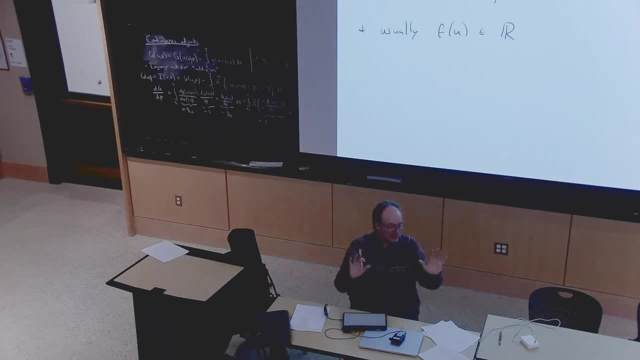 oscillate infinitely fast or they can blow up or do things like that. So if you want to do rigorous math with functions, you spend a lot of time kind of nailing down the space of functions that are not terribly behaved. I'm not, I'm not going. 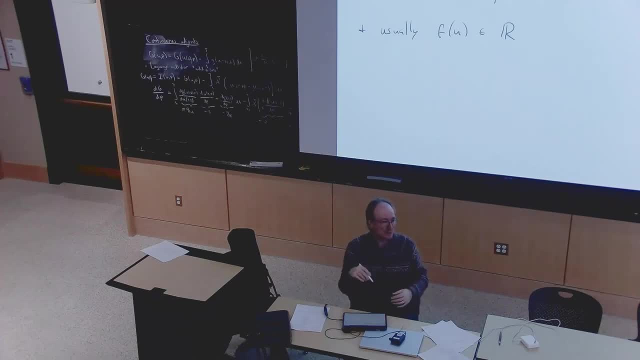 to do that. I mean, I'm just going to be kind of implicitly. I'm going to write down an integral of functions of a function. I'm going to implicitly assume that we're dealing with functions where that integral is defined. So you know. 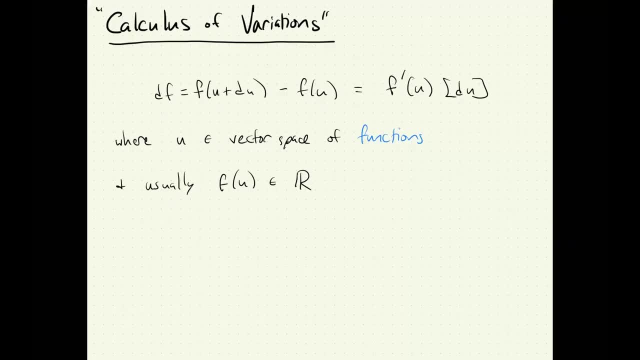 that's things like that, right So. so for let me just do an example, right So let's do u of x is a function you know from, you know zero to one, right, X is in. 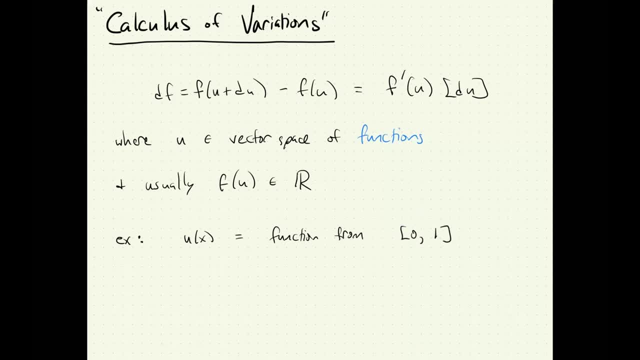 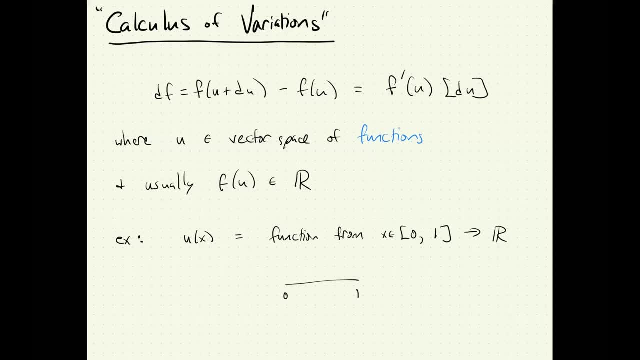 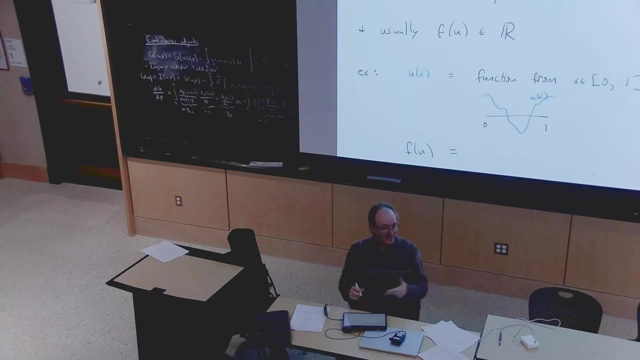 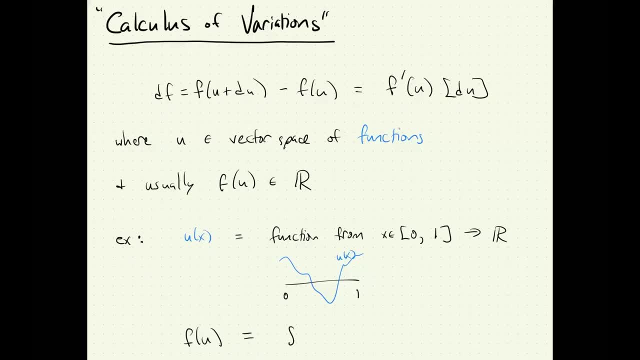 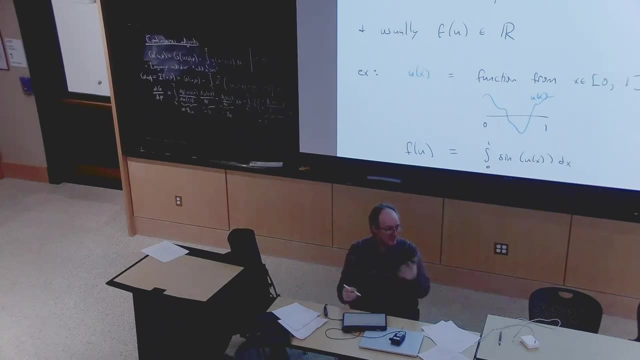 is is just integral zero to one of, say, sine of u, of x, dx. let's just start with right that takes in a function, gives me a number. technically it doesn't work for all functions. right, you could have functions where this, where this, this integral doesn't exist, or something like that. so implicitly, I'm limiting myself to the space of functions where the integrals work right and what I want. 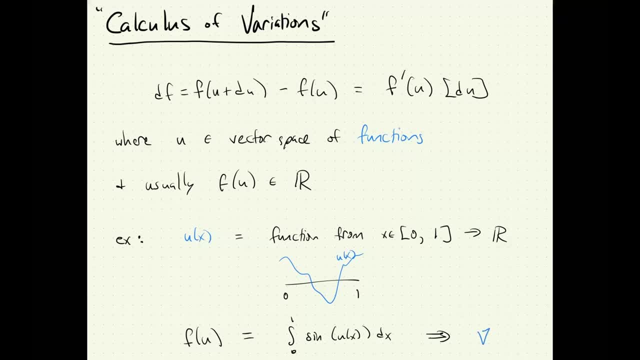 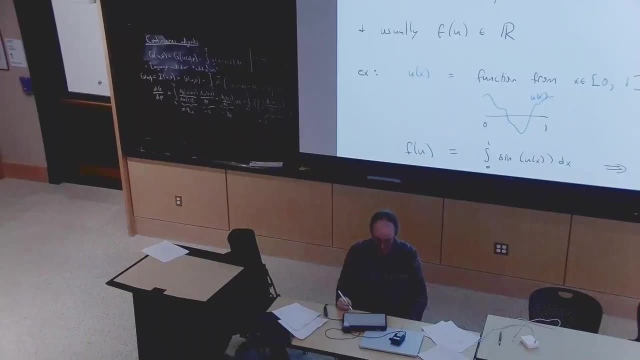 to do is find out what is the, what is the gradient of f right, what is and what is f prime also right with respect to u, of course. so now, with respect to a function right- and it's going to be exactly the same definition for it to take a derivative. to take a derivative, I just need to linearize. I need to ask: how does f change for a small change in the input right? linearize it. 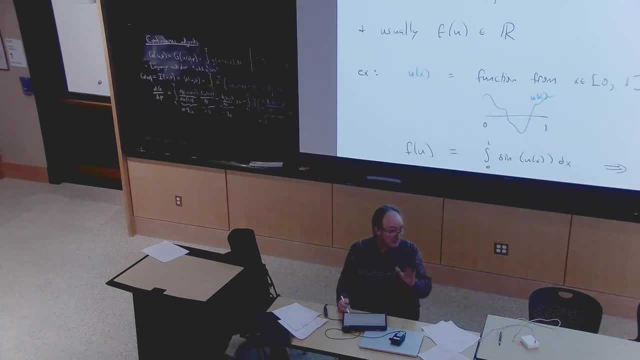 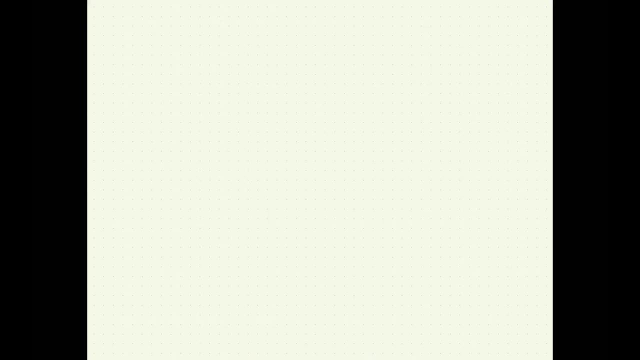 and then to get one step further, to get a gradient, I'm going to need a dot product. but let's do this before we do the, the, the gradient and the dot product, let's just linearize, right, so right. so we're going to take df, we take f of u. remember u is a function, by the way, this is sometimes called a functional. 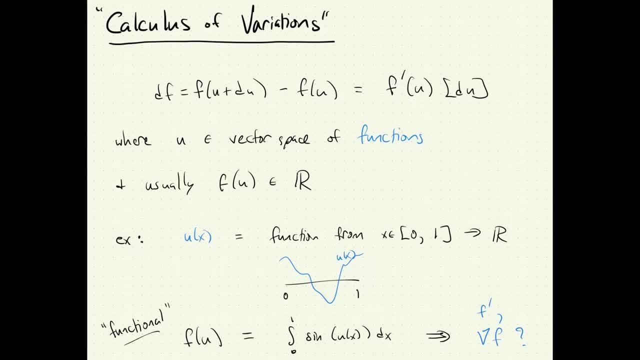 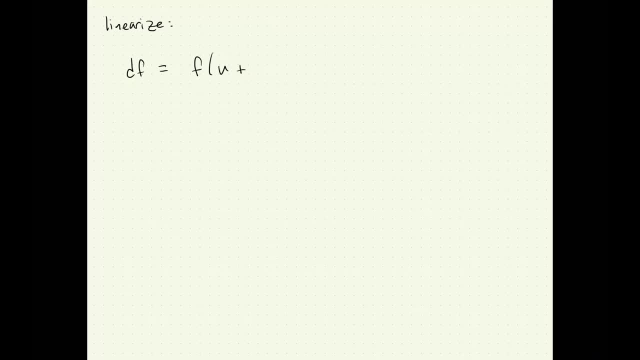 it's something that takes in a number, a function, and gives you a number, but sorry, and I'm going to, and here I need f of u plus du minus f of u, and the key thing to remember is that this is a function. u of x, that's a terrible x and this du here. 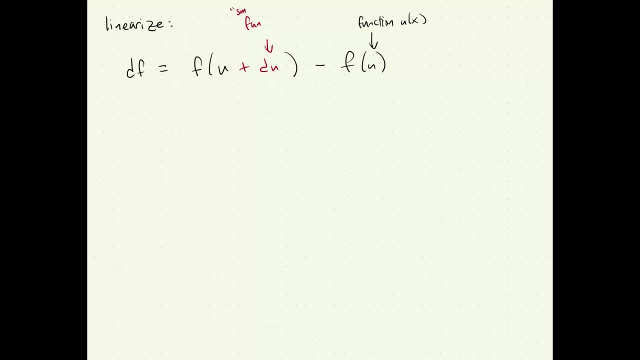 this is also a function. you can think of it as a small function. du of x. right, and as I said last last lecture, to get some notion of small we're going to need a norm of a function. but pretty soon I'll have dot products of functions, so I'll have norms as well. so let me sweep that under the rug. but it's just like a little perturbation, right? so you're taking, you're taking, you know, u of x. 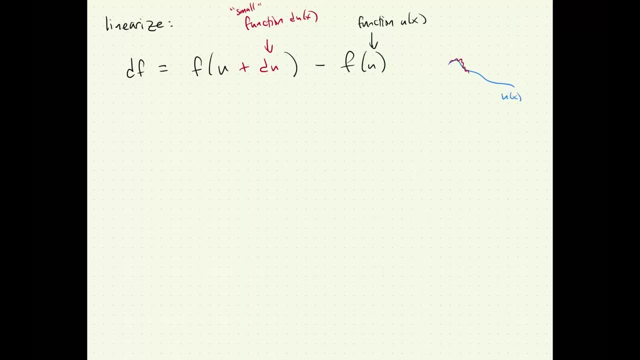 u of x and you're adding, you know, some arbitrary little change to this. this is a u plus du of x, right? so you're going to change, change that function by a little bit anywhere you want. it has to be small, and then we're. so we can drop terms that are that go like du squared right, and so what is this? so this is integral from 0 to 1,. 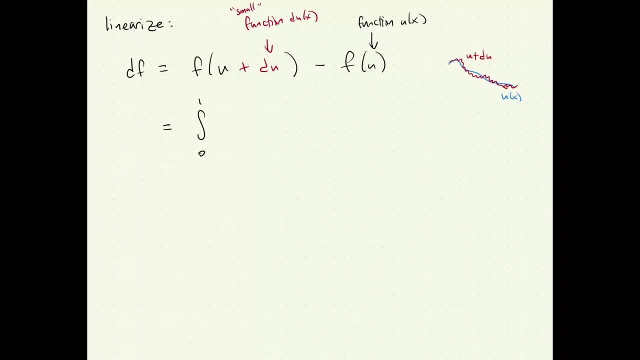 I said f was sine of u of x dx, so this is looks like sine of u of x plus du of x minus sine of x dx. I'm just plugging that into my f. my f was integral sine u, right, and I'm going to ask: how much does that integral change for a small change in u? and I want to linearize. 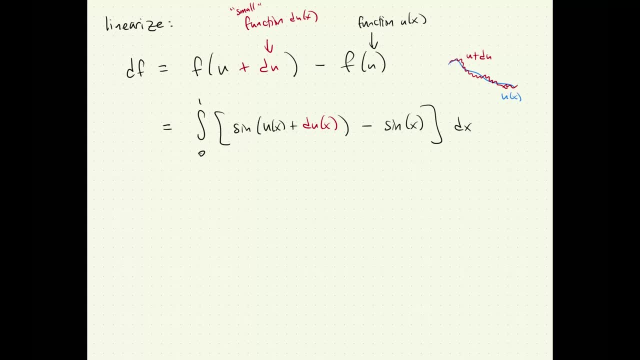 it right. so I want to write this as drop every term that goes like du squared or higher. so, and of course, the point is, all I need to do is linearize this, linearize the integrand right that thing sine, oops, sorry. and this is not sine of x, this is sine of u of x. 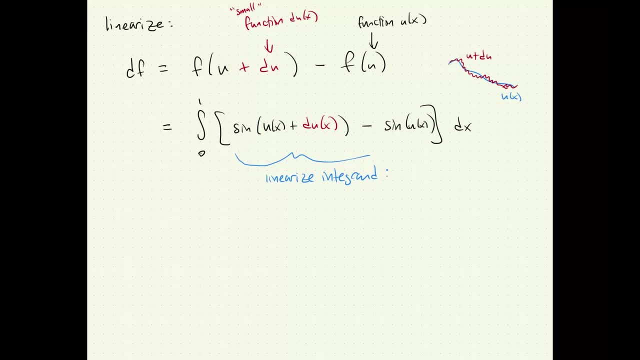 okay, so I want to, I want to linearize this. what is sine? so sine sine of u plus du, right, that's equal to sine of u plus the derivative, which is cosine of u times du, right? this is just because this is du of du is a function, but du of x is a function, right. 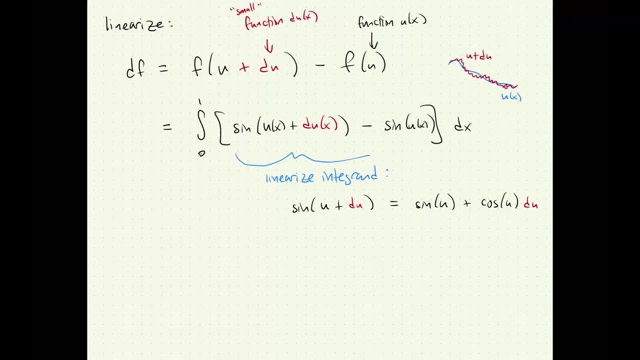 X is just a number right. At each X I have a small change in U of X, So this is just ordinary. you know, 1801, right linearization, or from lecture, one of this class right, Or this could be a, you know, yeah anyway. so this is just a number, ordinary linearization. 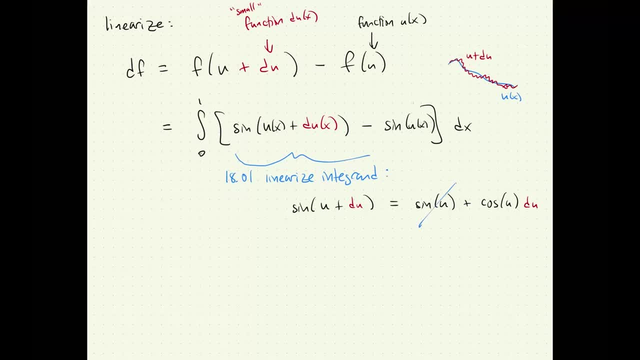 and then, of course, this term here cancels that term right. So what this is is integral 0 to 1 of what's left cosine of U, of X, DU, DX, and this is exactly this is a linear. 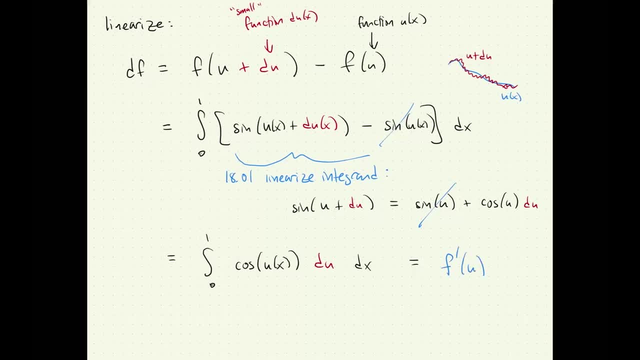 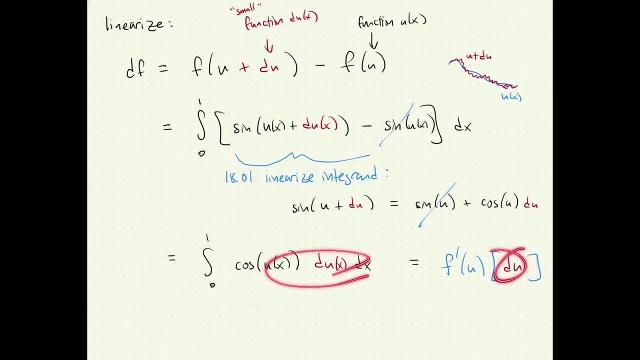 if I double this, it doubles the integral. Like, if I add two things here, it adds two things in the integral. So this is a linear operator. This is we're done From that takes DU in and it gives you out a number. right, This is my DF. 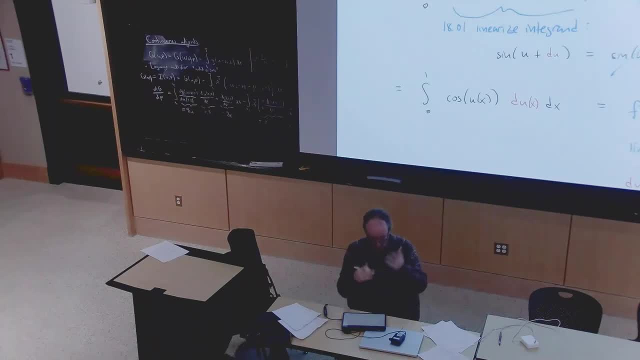 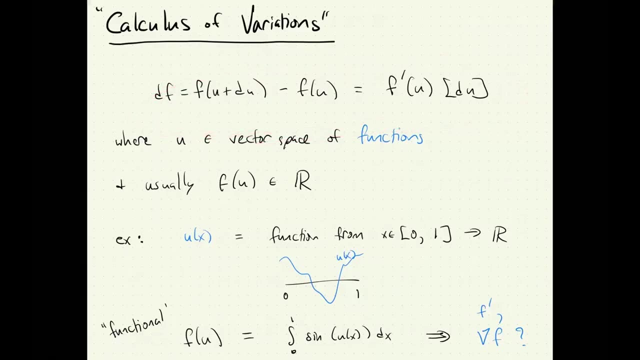 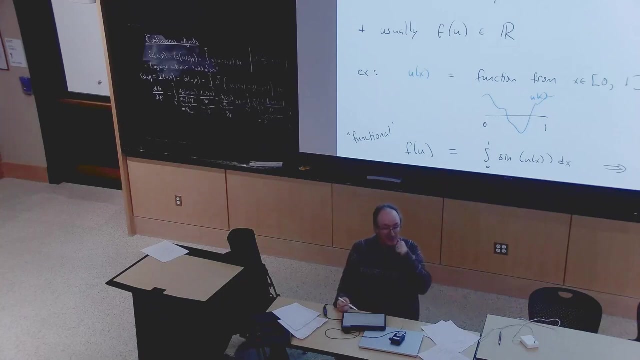 So you know, once you get used to this as being, you know the definition of a derivative right and you can always fall back on this When U is some crazy object matrix function. whatever, as long as it's a vector space or technically a Bonnock space, it has to. 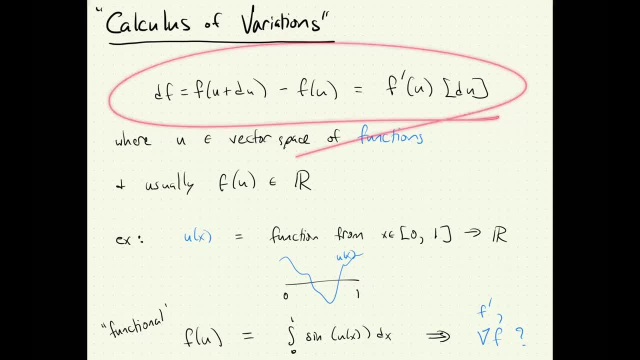 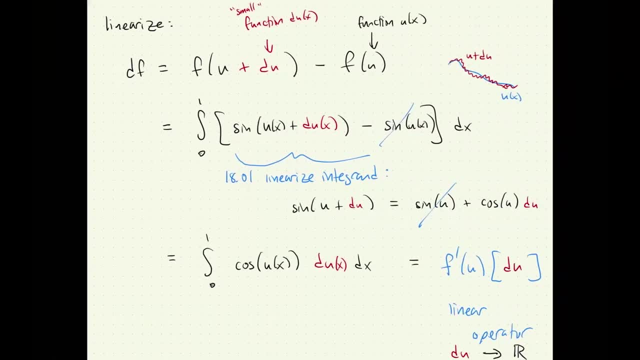 have a norm, then you can define the derivative as the linear operator. that gives you the first order change right. So, as I said, technically you know we're dropping terms of you know little O, of DU right, Terms that go to zero faster than DU here. So to have to make that precise, you 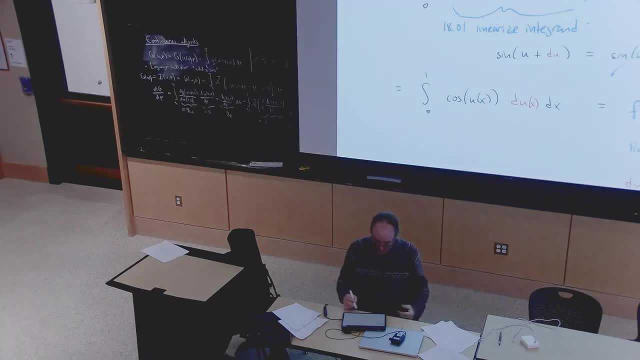 need to have a norm. But anyway, this is a function that takes a vector, my function- I'm thinking of it as a vector space, a vector in, and it gives you out a scalar. So I should be able to write that linear operator, this linear form, as a dot product with some sort of 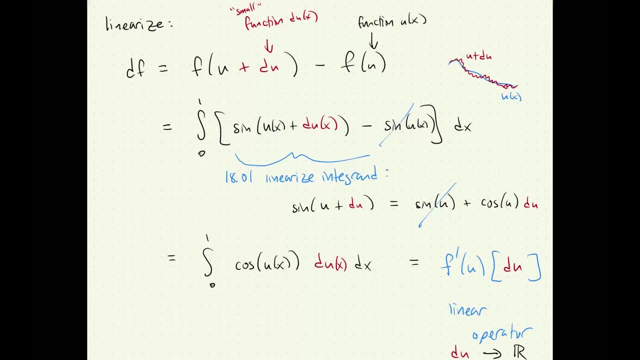 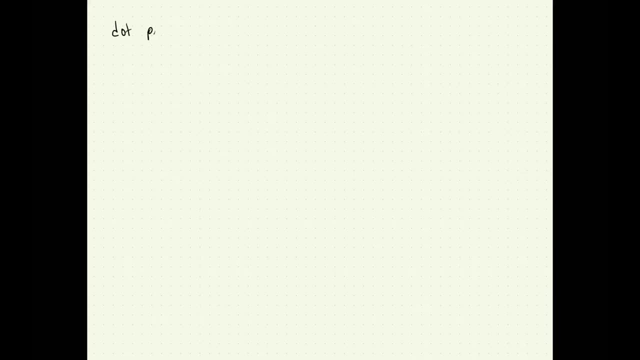 something. So for that also I want a dot product which will give me a norm. So let's just remind you- hopefully you've seen this before in 1806, or in some other linear algebra dot products of functions, right? So yes, 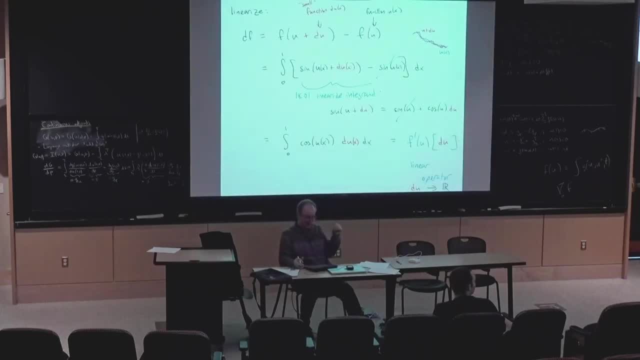 I have a quick question. I guess one takeaway that I have so far is that this derivative is a linear operator right, And so you know, when you have a vector space you have to have something in the dual space. so it's saying that the input will be a function. 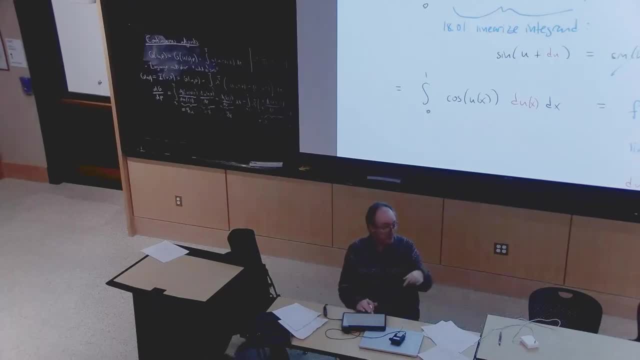 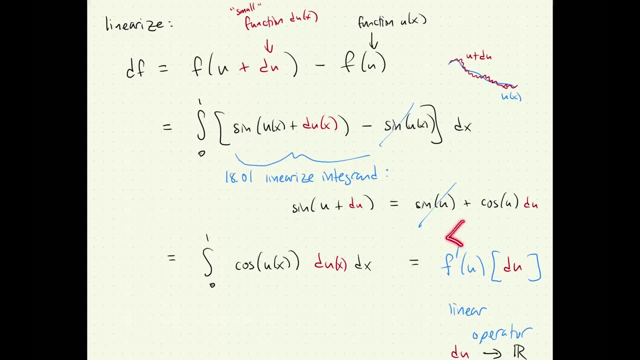 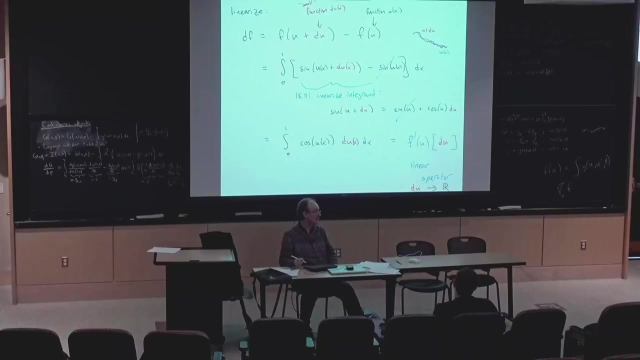 Yeah, Well, if it's, if the output is a scalar right, Yes, Yes, So this is exactly something in the dual space Physicists would call this a bra. Well then, if this is a function, would I expect that the output is a distribution of? 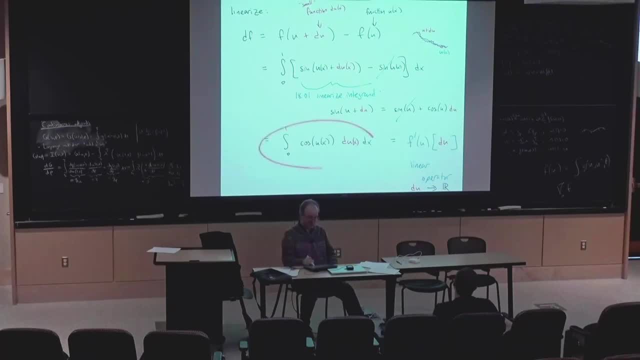 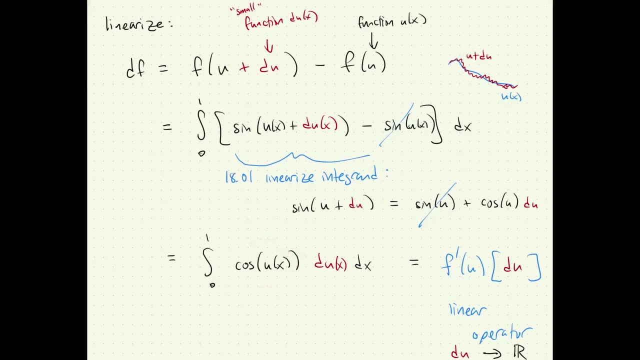 measures. Should I think of this as like the cosine of the density of that? Yeah, Yeah, this is a measure, Because that, that, that, that, that, that, exactly this is the density of that measure. Yeah, Absolutely This. this takes the measure. 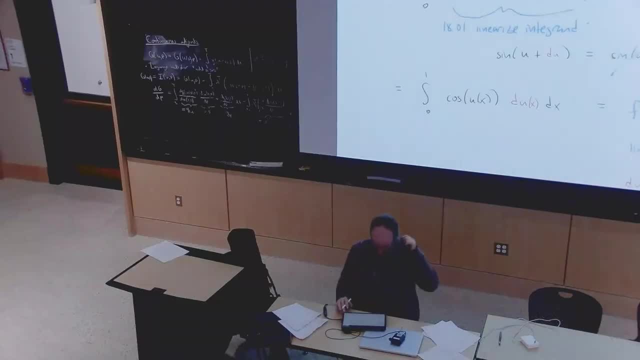 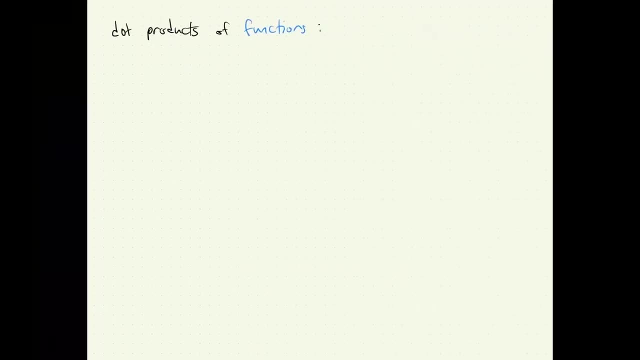 of that function Exactly, Yep. So it's all sorts of you know. you can think of this as a linear form or something in the dual space, or a covector, this vector space, right, I want to say it's a little bit informal in terms of those abstractions here And as I 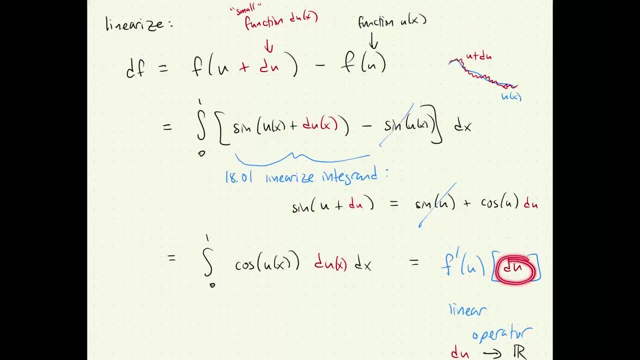 said. you know, technically speaking we have to restrict ourselves to not all possible functions here. There have to be functions where this integral is defined, so there can't be functions that blow up. So you know, I think that's a good question And I think 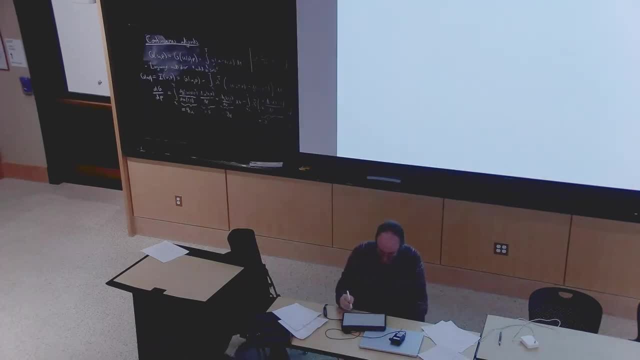 we can go on. you know, you know, I think we're getting pretty close to the fact that. I think you know, that's a very interesting thing. okay, That that's something that pure mathematicians worry about, that physicists and engineers. 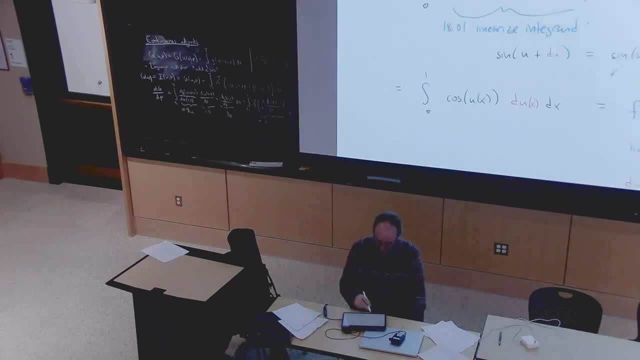 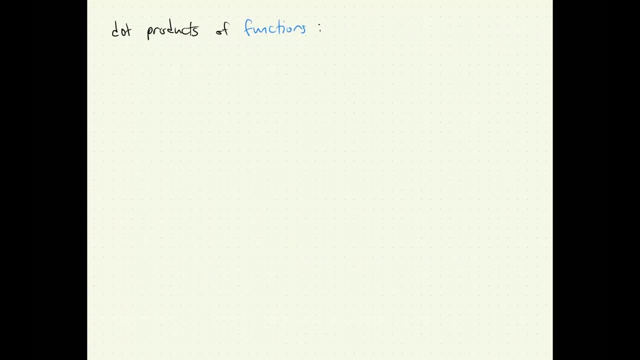 don't, because you know the, the functions. basically, if this is a physical context, again implicitly you're dealing with functions where these things are defined Like you know you'll. you'll only really worry about ruling out those crazy functions if you're. 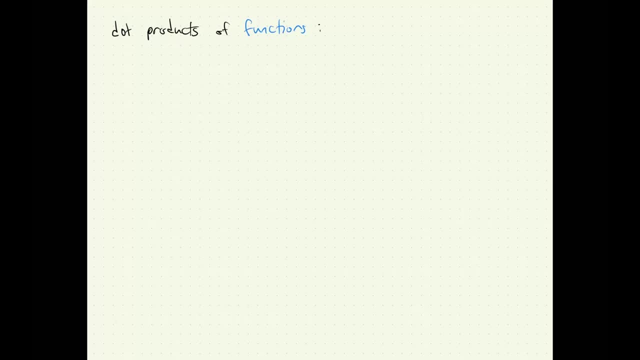 if you're doing pure math, that's unmoored from reality. So okay, So, dot products of functions. So so you know, if you take a dot product of two column vectors, the standard function is, you know, a simple data function, right. 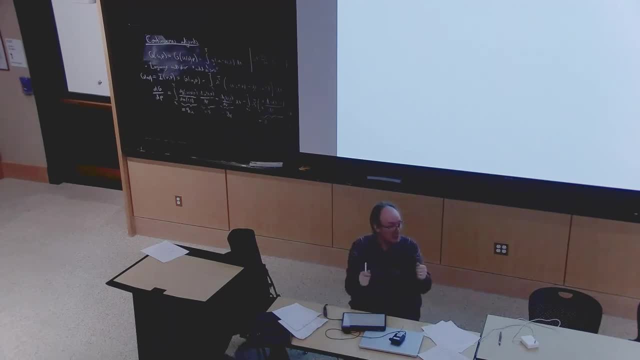 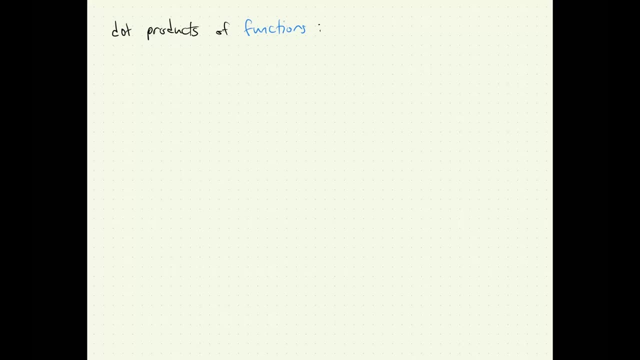 column vectors, the standard. there are many dot products, but the standard one, the Euclidean one, is you just multiply the components and add them up. So if you think of two functions, you know u of x and v of x. you know on x in 0 to 1, then the sort of the Euclidean 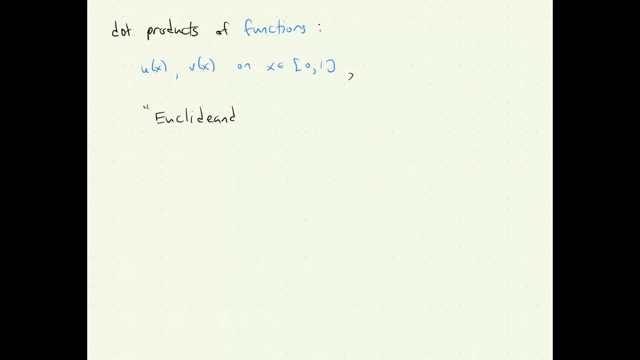 dot product, the sort of the obvious dot product, the Euclidean inner product. right should be to multiply the components and add them up. So the components. if you think of these as column vectors, they're like infinite dimensional column vectors. the components are the values. 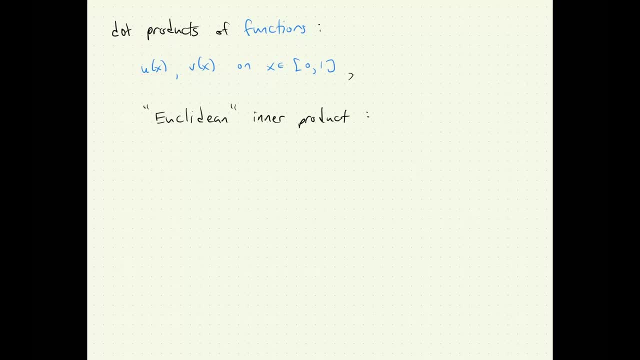 at each point. So multiply, you want to. basically, what you want to do is multiply u of x times v of x and add that up for all the x's. and the analog of adding it up, you know, you know, is an integral. That's our u dot, v. So we can do, and of course this is not the 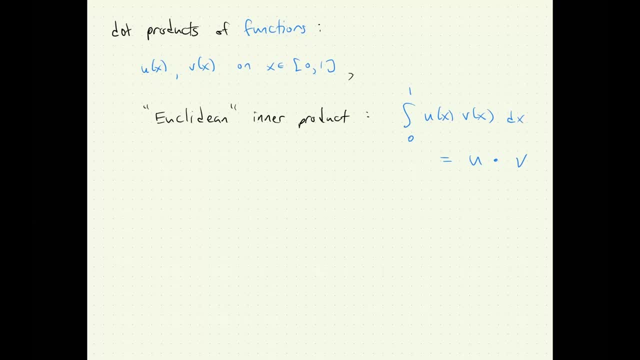 only possible dot product, but this is the most obvious one, the first one that you typically reach for right. So once you have a dot product, then of course we have a norm. So if you want the norm of u, that's the, that's the square root of the integral from 0 to 1 of u, of x. 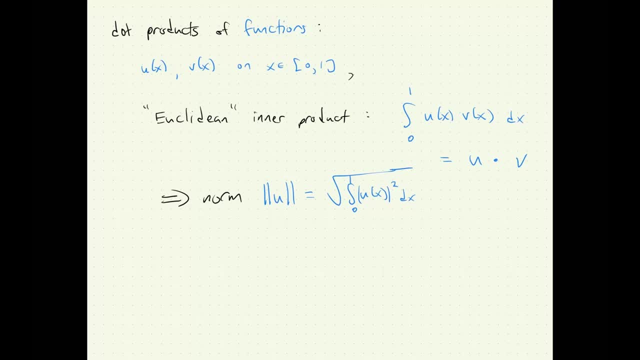 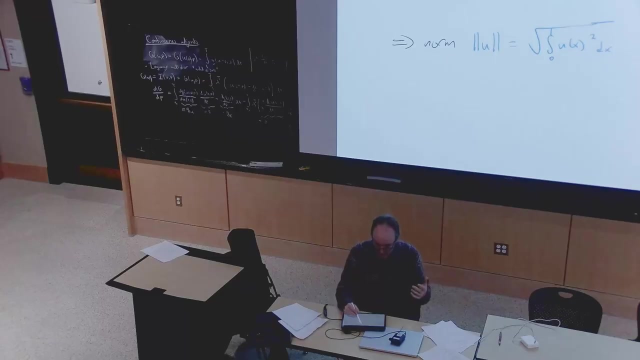 squared dx. I guess I don't need absolute values here, because everything is real right now. If it, if they were complex, I'd be putting complex conjugates over one of these, but So I let me remove my absolute values there, just for I don't need them right. So, and this is, 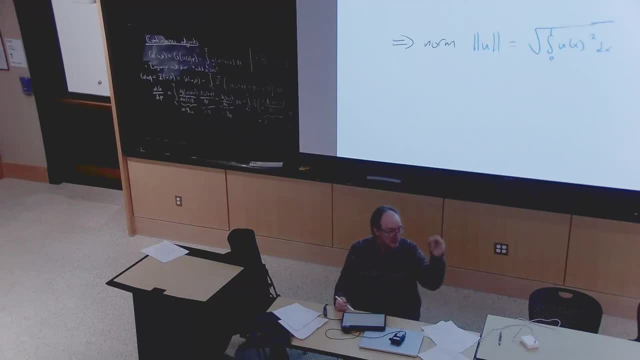 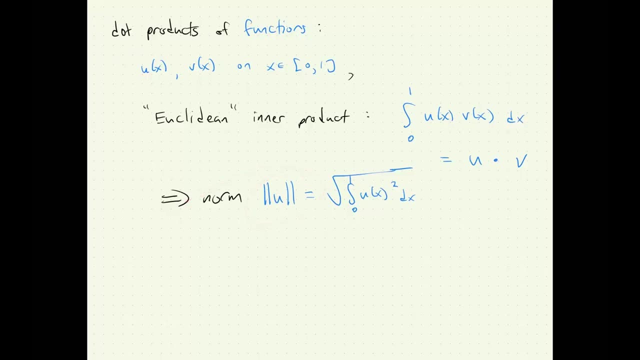 and once we have the norm, then then that's the precise sense in which we're dropping terms that go like du squared, right. So. so we're going to drop, drop terms that go like the norm of du squared and higher. 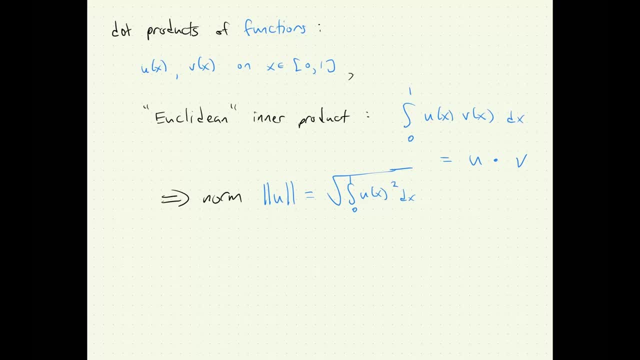 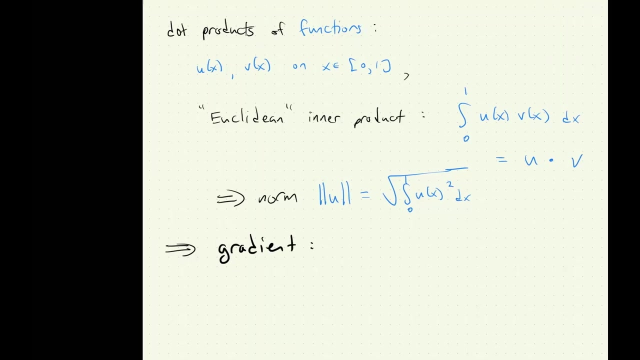 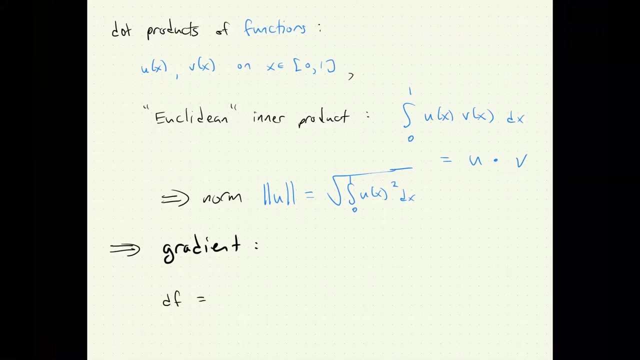 Actually anything higher than linear right. And once you have this, now we can compute, we can find the gradient right. Because what, what was our df right? df which was f primed of u acting on du right. 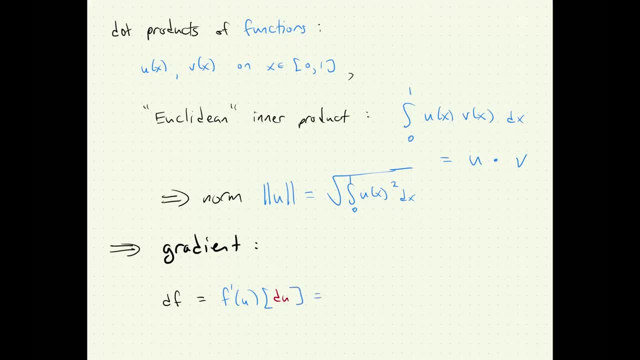 We said that was integral from 0 to 1 of of what is it? cosine of u of x times du, of x, dx? right, We want to think of this just. our generic definition of the gradient is when you have something that takes a vector, random scalar out. the first derivative had 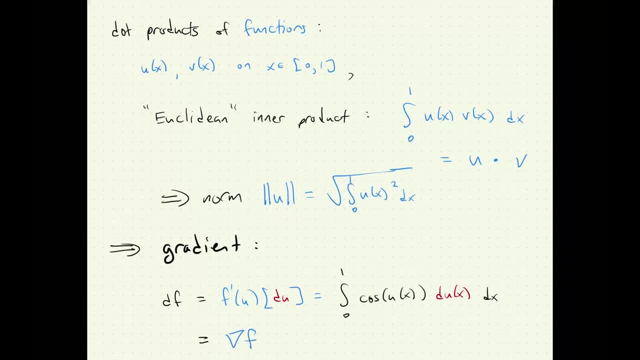 better be the dot product. Okay, Okay. So what is the gradient of the gradient with du? And if we just just by inspection, right, this is here, this is our definition of a dot product. So what is the gradient? 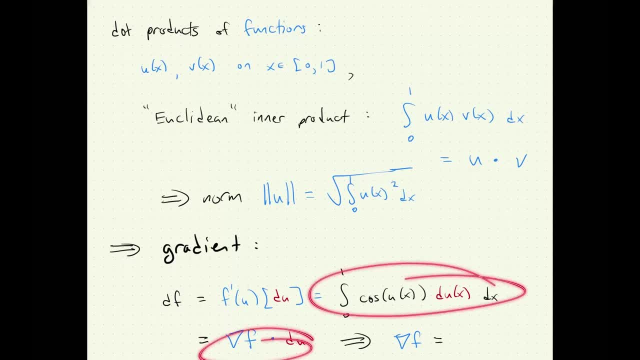 It's what. what would I take the dot product with du to of To get to get this Cos of u, Cos of u, exactly. So it's, it's, it's a function, it's just cosine of u of x. 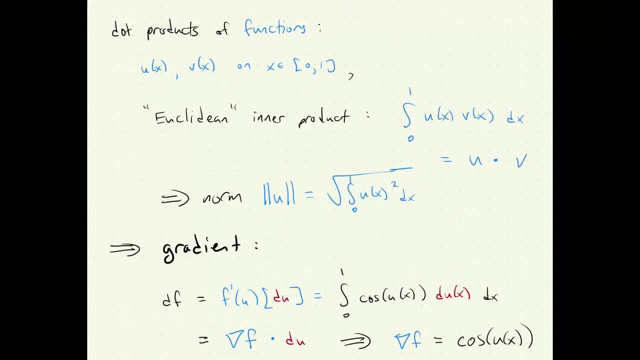 By the way, in this, this context, this is I'll, this, this is called. this is sometimes also called a Freshet derivative right. I, I mean Frechet derivative technically refers just to this general notion of if you have any. 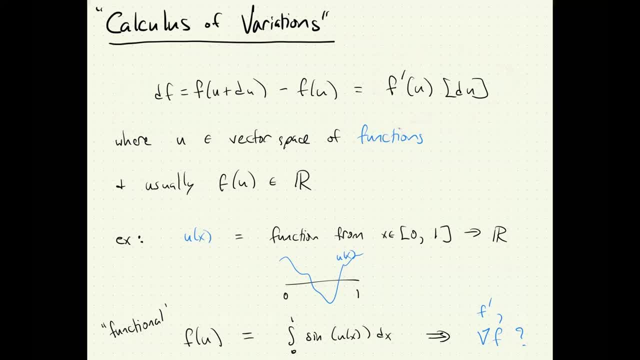 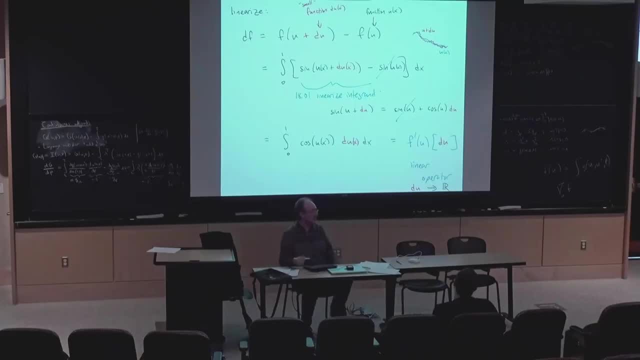 Bonnock space. the Frechet derivative is the linear operator that does this. But most often you see this coming up in the context of vector spaces of functions and that's where they use that terminology. For everything else people just say the derivative. It really. 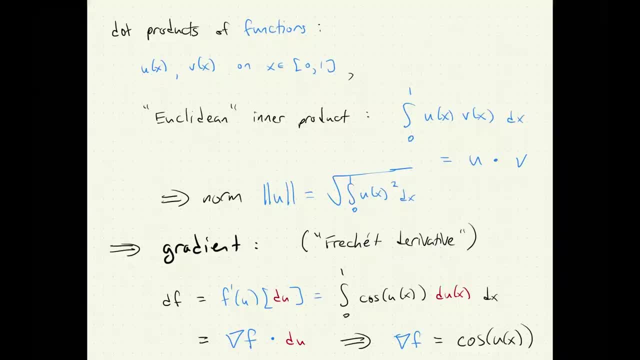 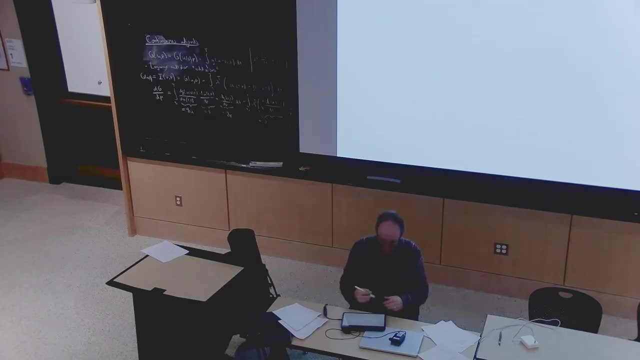 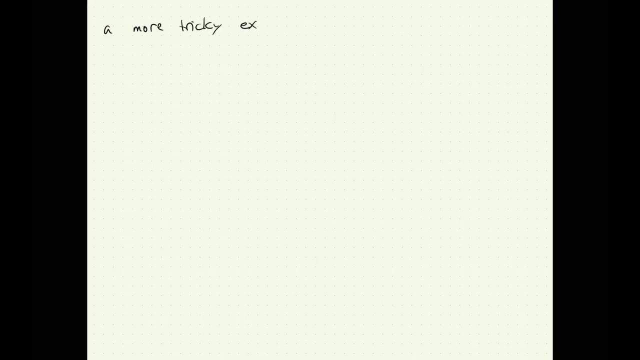 is just the derivative, but that's it. This is a gradient. So let's do a more complicated case. So let's do another example or a tricky example. Suppose that f of u – so we're still going to be …. de bu孱 u. 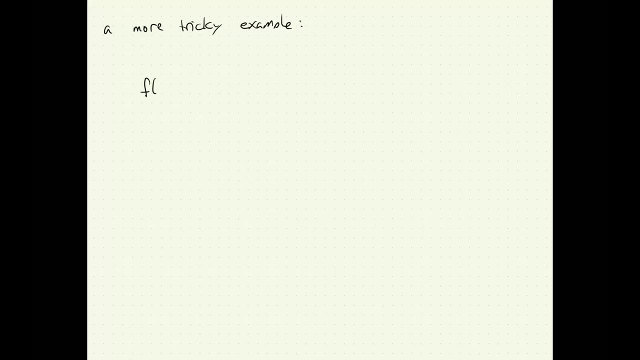 de f …. de f? u …. de f functions from 0 to 1.. Suppose it's the integral, from 0 to 1, of the square root of 1 plus u, primed of x squared dx, where this is just the derivative, The ordinary du dx, the 18 to 1. 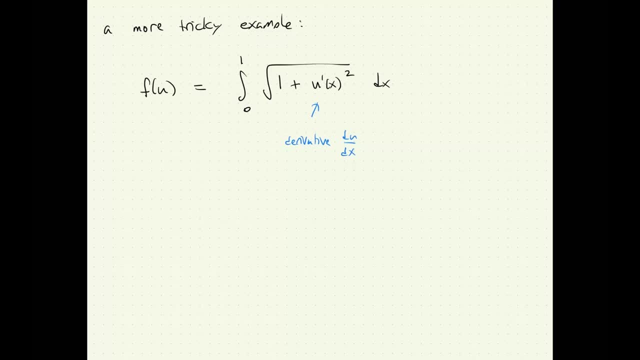 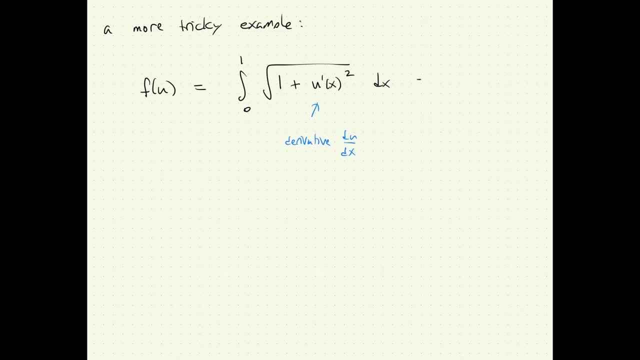 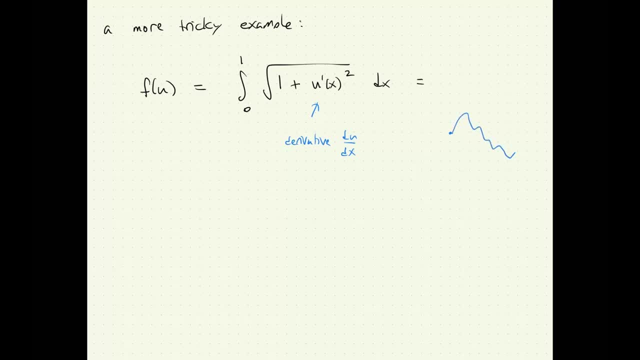 that. here's u of x. What is this quantity that I've just computed here From first year, calculus? there's an important name of this. yeah, u of x. It's the length, It's the arc length. right, It's the length of the curve, The arc. 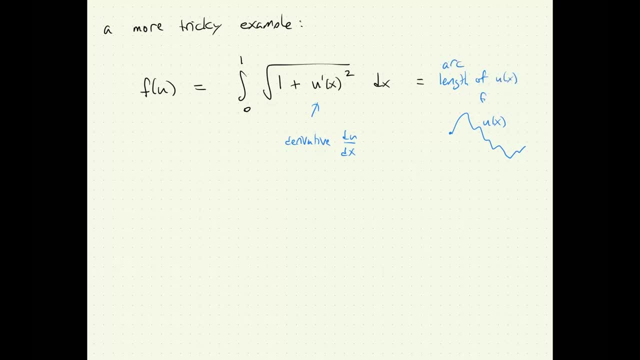 length of u of x from x equals 0 to x equals 1.. That's what this quantity is. If you multiply through by dx, this is basically square root of dx squared plus dy squared. If you take each little line segment here, it's the length of that little line segment that you're adding. 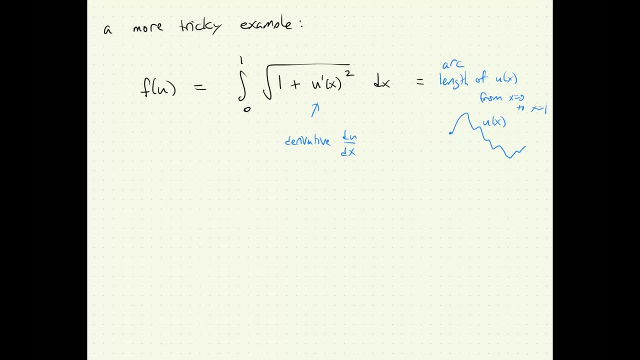 them up. Okay, So now let's think about the derivative. Okay, So now let's take f of u and we're going to add a little change to u right Subtract f of u. It's always good to just fall back on the definition, the most basic. 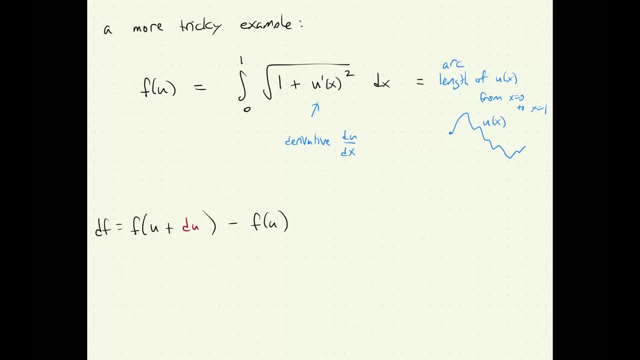 definition. Okay, we're in doubt of what to do. We're going to just add a little change. And what's this going to be? So let's just: it's the integral of from 0 to 1, the square root of 1 plus. 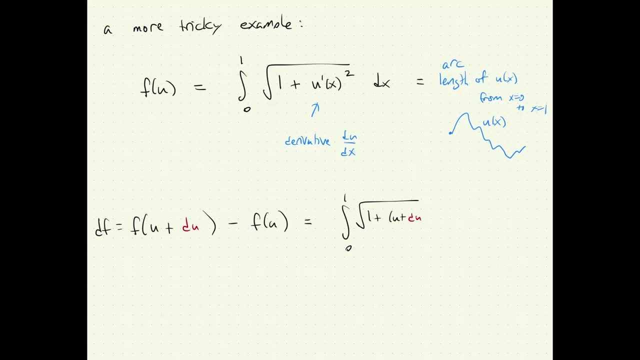 u plus du primed squared, minus the square root of 1 plus u primed squared. So again, we just think so. now we have to tailor expand this. But now we have to assume that du is now a differentiable thing And its derivative is getting smaller and smaller as well. So 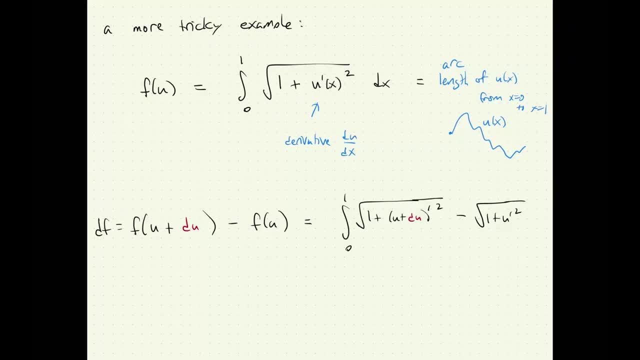 I can do this kind of expansion, first order expansion. So what is this? So it's the if I have, let's see, if I have 1 plus v plus dv squared, what's the Taylor expansion of that? That's 1 plus v squared. That's the first term And the second. 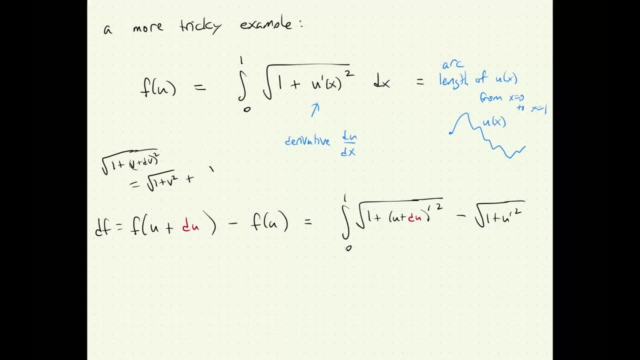 term is the derivative with respect to v, which ends up being v over square root of 1 plus v squared times dv, And I kind of went this through that a little bit. This is, but this is just 1801.. This. 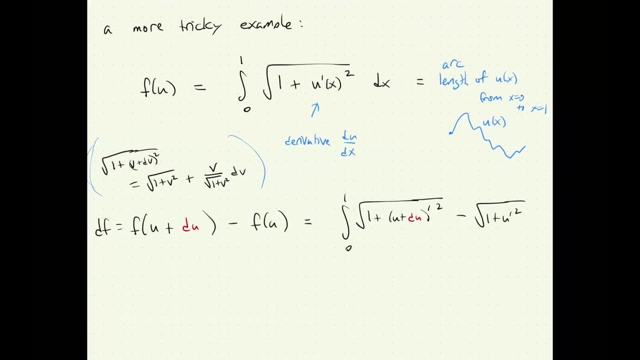 is just 1801, right, so plus right. This is this: is this function, for dv equals 0.. This is the derivative of this right. So when you take the derivative of the square root, it's 1 half 1 over the square root right. But then there's a derivative of this. 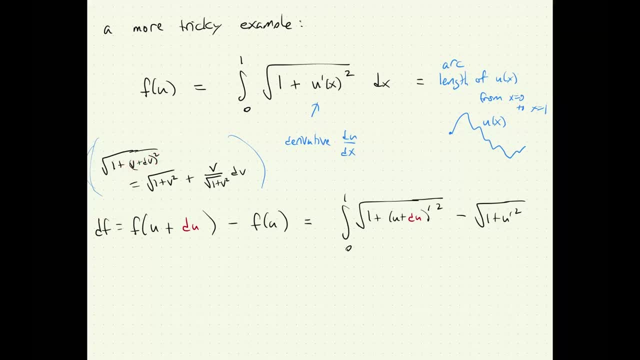 which gives you a 2v on top. So the 2 cancels the 1 half, right. So this, so just, so, just Calculus, expanding everything to first order in du and also du prime, so dropping anything that goes like anything with a du, whether you take a derivative or not, squared, we're. 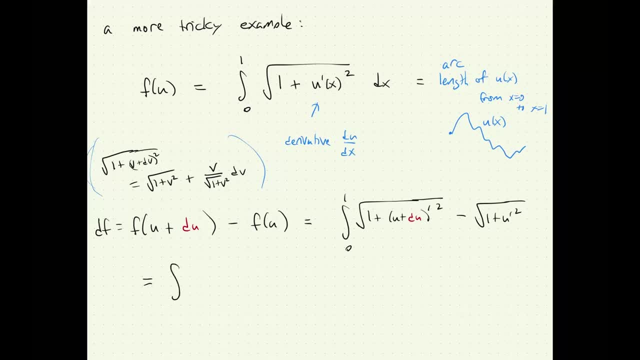 going to just drop. This is the integral of that second term, which is u over square root of 1 plus u squared times. sorry, and du that's primed divided times, du primed dx. So this is a linear operator. 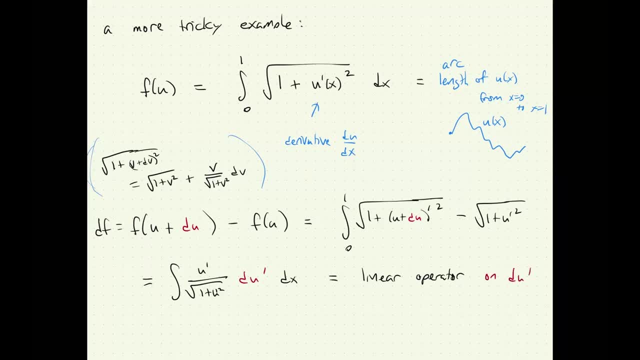 But it's acting on du primed, not on du per se right. I mean, the derivative is a linear operator on du, but I'd like to write it directly in terms of du right, Because I'd like to write it eventually as a gradient, write it as a dot product of something. 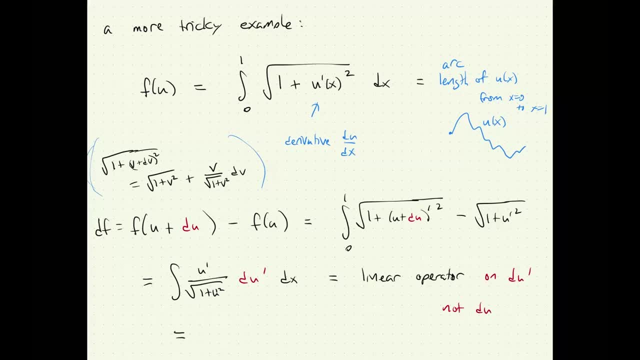 with du. So what I really want to do is write this as a dot product of a gradient dot du, and somehow I have to get a du and not a du primed. So we just saw this in the first hour. If you have an integral and you have a term that has a derivative and you don't want the 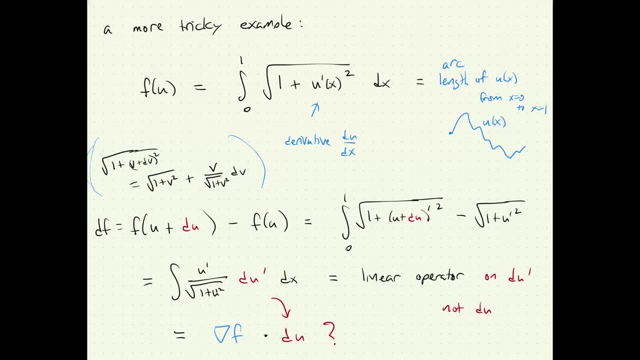 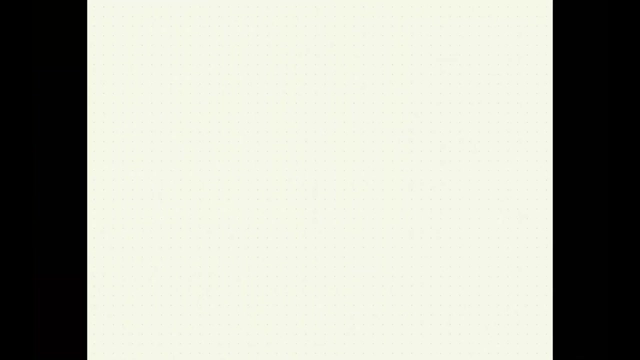 derivative. what do you do? What can you do in first-year calculus to get rid of a derivative on a term in an integral Integrate by parts? All right, All right, All right. So what do we do? So that whole thing? let's see df. there is a boundary term that looks like u primed. 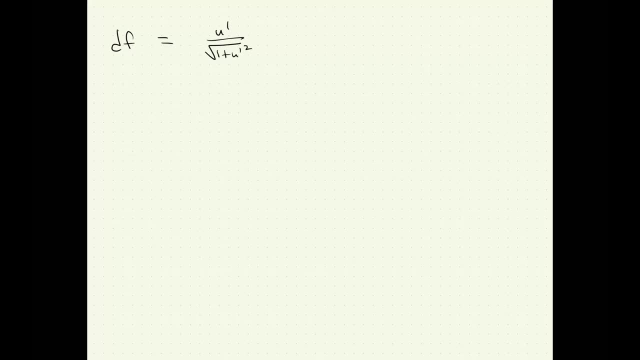 over square root of 1 plus u primed squared times du at the boundaries 0, 1.. And then you have a minus sign and an integral from 0 to 1 of du. All right, So we take this whole thing: prime du and then times dx, right? 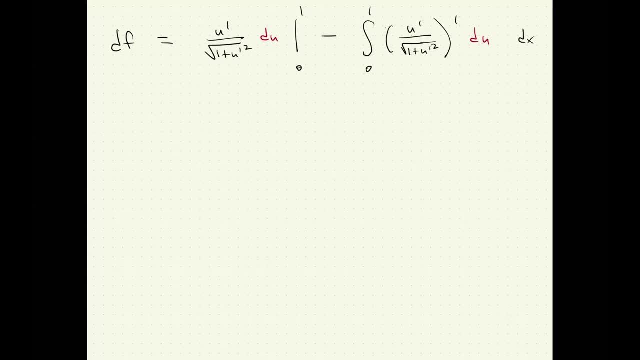 All the u's and du's are functions of x. So, to go further, I mean, this is it. This is the linear operator. All right, You know, this is now our, Our f prime of u acting on du. This is a linear operator acting on du and there's no du primes here. 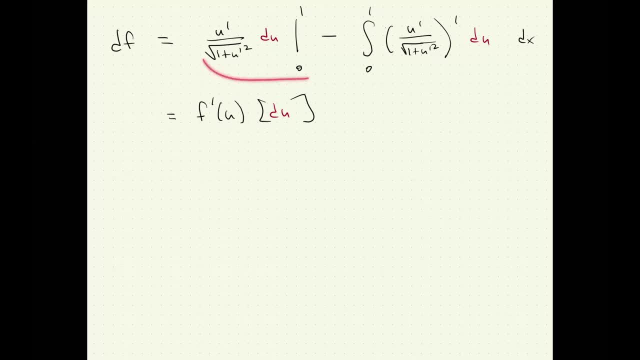 This is nice, But it has these. These boundary terms are kind of annoying, right, But usually in the context where I'm interested in this, I'm actually going to set some boundary conditions. So, in particular, suppose I want to fix the endpoints of my u. 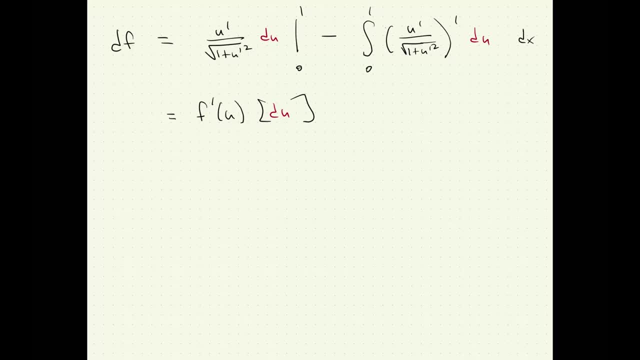 All right, And I want to find the, The curve that has the minimum distance from one point to another. Of course that's going to be a straight line, right? But suppose I didn't know that, right? So, And this is: 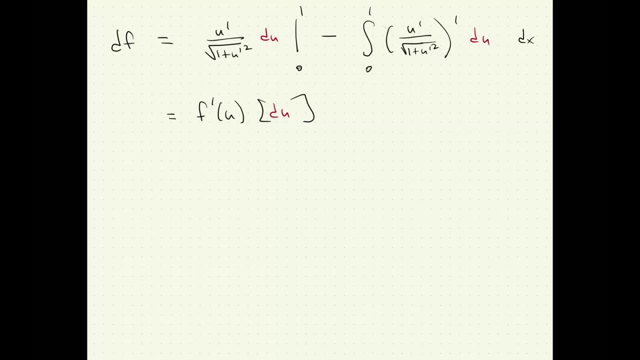 This is a simple problem where you know the solution ahead of time. but the more complicated things you won't know that All right. So I want to Suppose we want to fix. To fix, Let's just even say u of 0 equals. 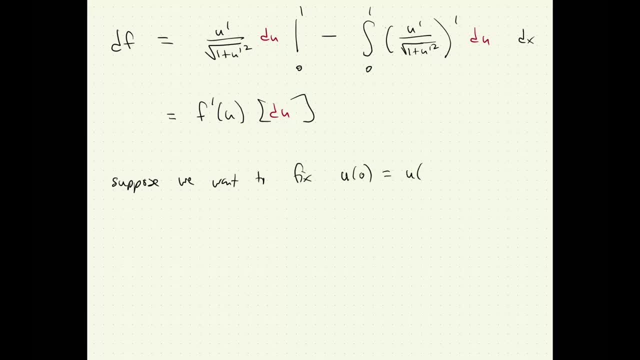 Let's just even say: u of 0 equals. Let's just even say u of 0 equals 0 equals u of 1 equals 0, just for simplicity, right? And so that's. And now we want to find the u that minimizes the arc length f of u, right. 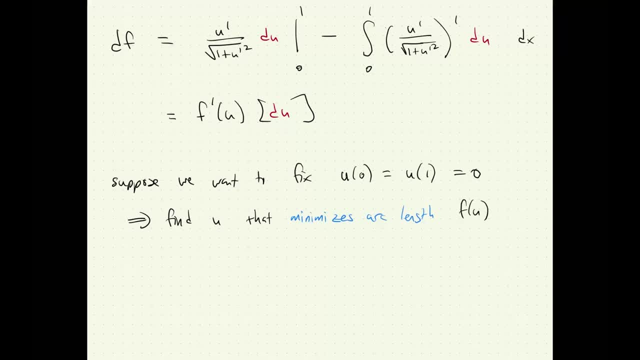 We know, probably it's a straight line from one point to the other, right, But let's pretend we don't know that. So, So what we want, If you want to minimize something, what you want is for the gradient to be 0, right. 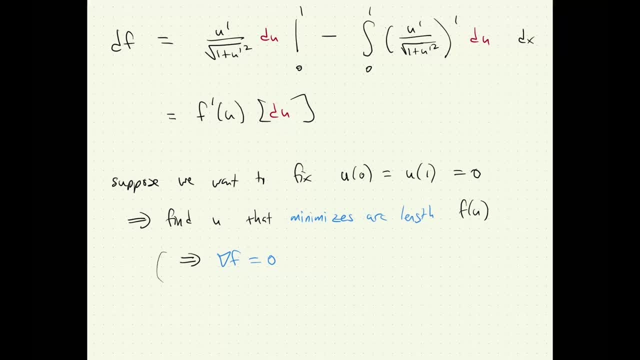 So we're going to need to take a gradient set equal to 0 in a minute. But if we fix the endpoints, we're going to want du also, at 0 or 1, to be 0, right, If we fix them at 0.. 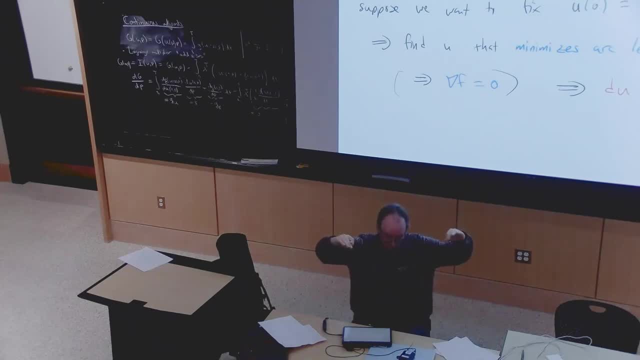 Because if we start with a vector space of u's that are 0 at the endpoints and we want to look at not all possible perturbations but perturbations that keep those end fixed, Or if I kept the ends fixed at some other point still I would want to look at- not 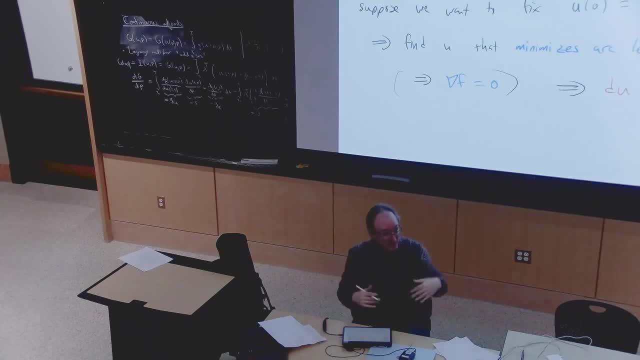 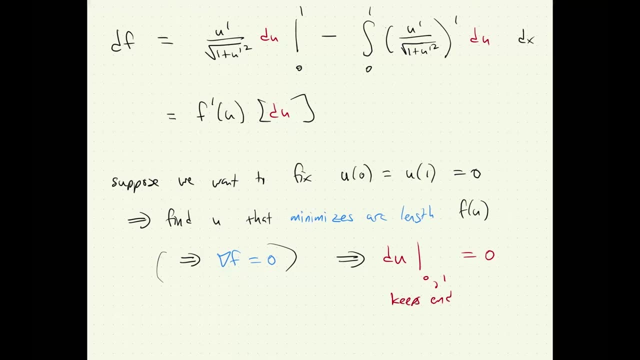 all possible perturbations, right. I'd want to look at the perturbations that keep the ends fixed so that the? u is 0 at the ends. So this keeps the endpoints fixed, right. And then what happens? What happens is that that boundary term disappears, right. 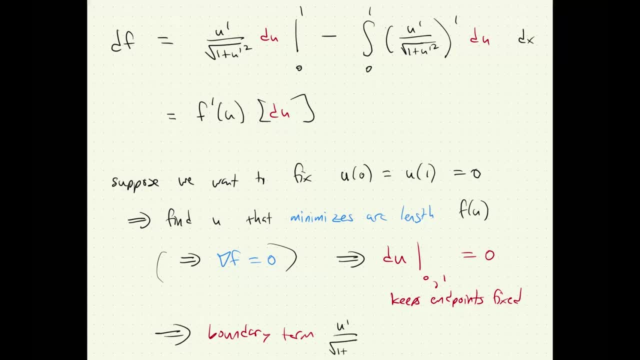 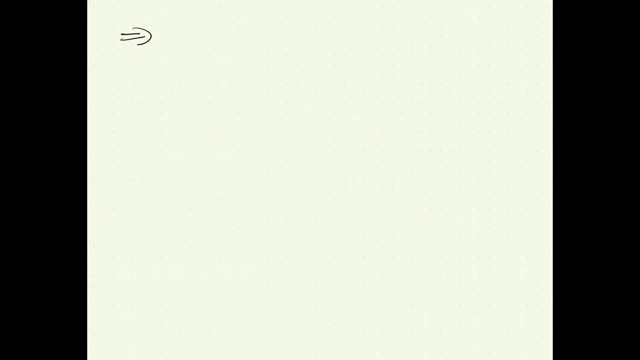 Our What was it? u primed over square root of 1 plus u prime squared du taken at 0, 1.. This is now just 0, right, Because you fixed the endpoints. So now Df is just integral 0 to 1.. 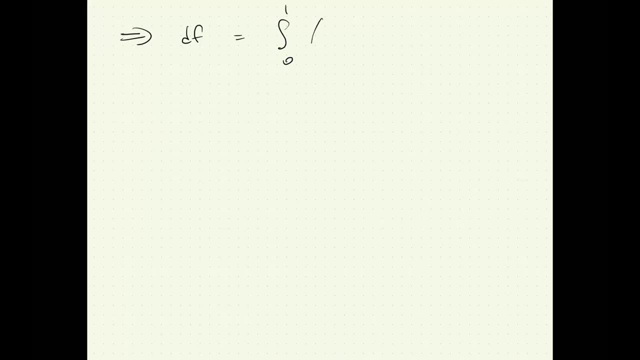 So what happens? What happens? What happens? We get 1 of u primed over square root of 1 plus u prime squared primed times du dx. So our gradient is just this thing here. right, It's the thing we're taking with the dot product of du with to get the solution. 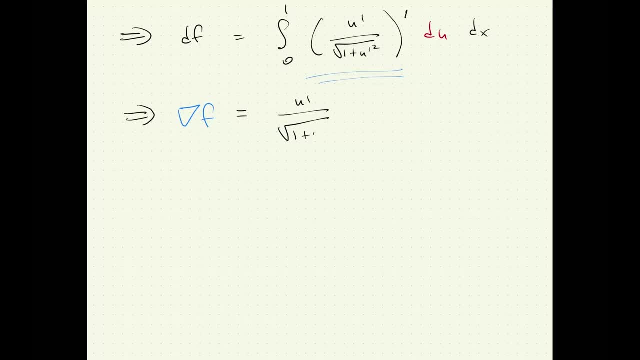 So it's just u primed over square root of 1 plus u primed, squared primed. Okay, So now I don't know if you can see this- It's just u primed over square root of 1 plus u. 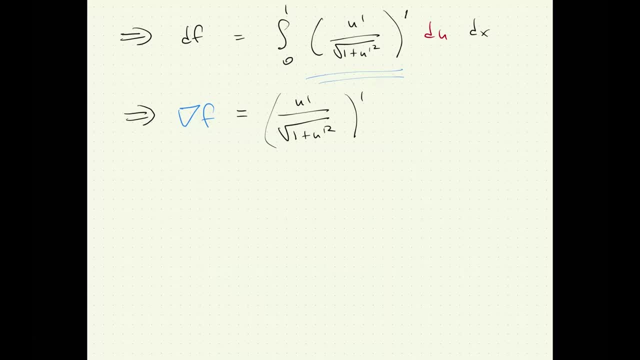 Does everyone see that? So this is the. This df had better be the dot product of grad f. with that, With that grad u, I integrate by parts. I turned my u primed into a du. I set boundary conditions to fix the boundary, so the boundary terms disappeared. 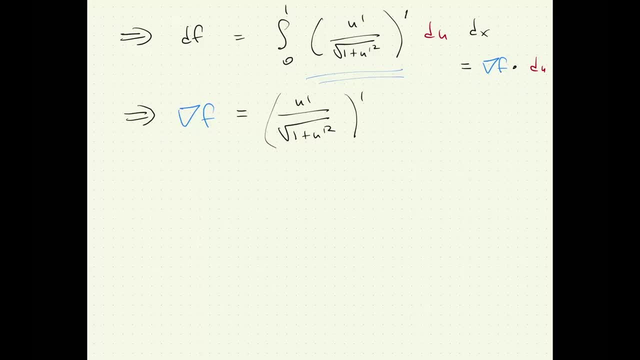 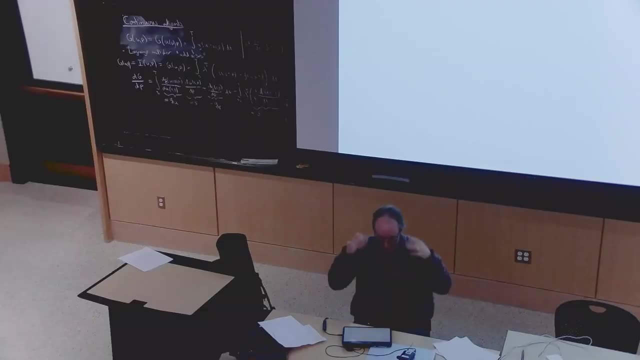 What I have left is just a dot product of this with du, so I can think of this as the gradient right, And if you're at a minimum it's the same Right. So you don't know what it is same for the same reason as in 1801 and 1802 and so forth, at a minimum the gradient has. 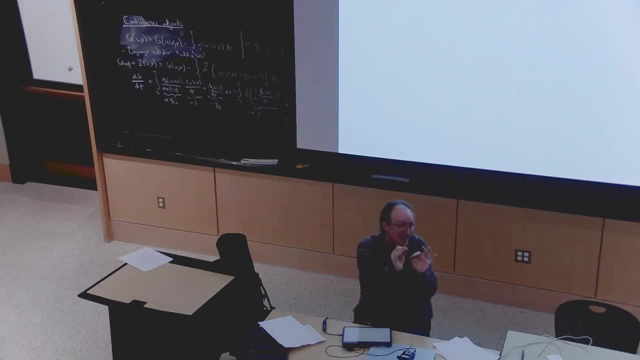 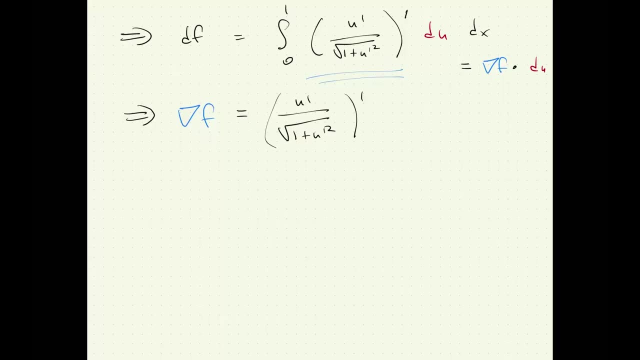 to be zero, Because if it's not zero, you could move in that direction and make it bigger, or move in the opposite of that direction and make it smaller. So this has to equal zero at a minimum. And so now let's just. I need to work out. okay, now it's a little. 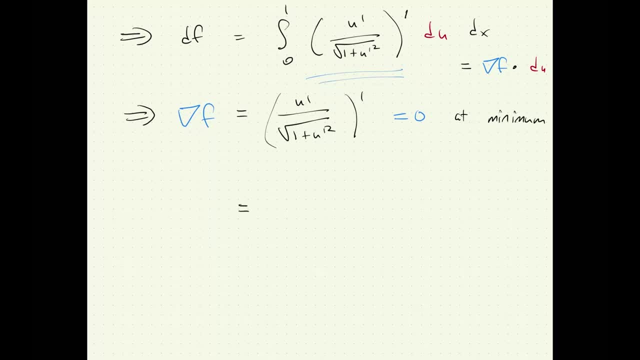 bit of a calculus exercise. What is the derivative of this thing? Okay, so now it's quotient rule, right? So this is going to be quotient rule. So in the quotient rule on the bottom you get that denominator squared. so you get 1 plus u primed squared, the square root squared. 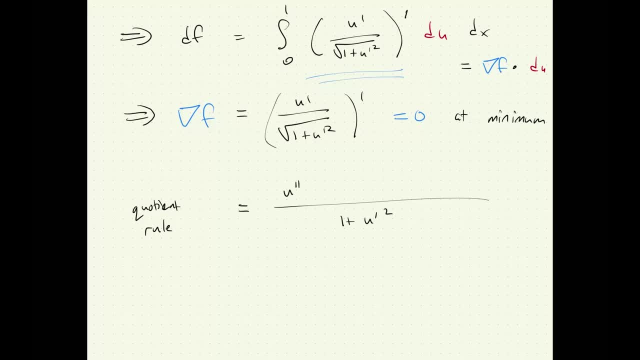 On the top, you get the derivative of the top, which is u double primed times the bottom square root of 1 plus u primed squared. Okay, And then minus the top times the derivative of the bottom. And we just did that, The derivative. 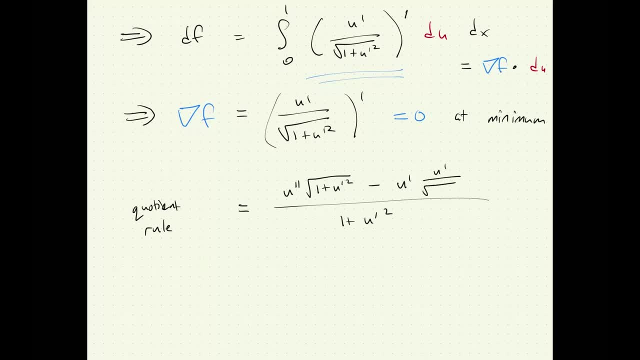 of that square root is in fact u primed over square root of 1 plus u primed squared, I think Did I make. hopefully I'm not making any mistakes here. Okay, so now, if I want to put this over, try this a little bit. This is 1 plus u primed squared. I'm just 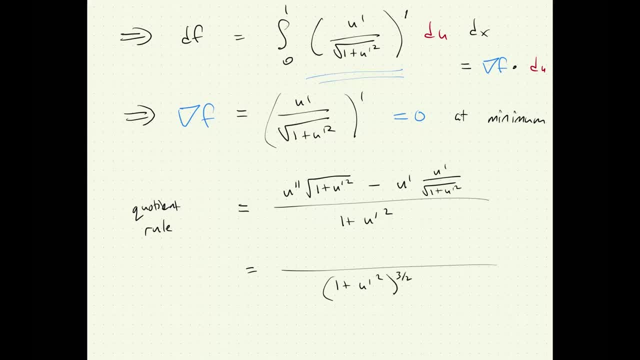 going to put three halves on the bottom, So I'm going to pull this term and put it on the bottom. so I'm just going to multiply and divide by square root, Okay, And what you get is the? u prime times 1 plus u prime squared minus u prime squared. 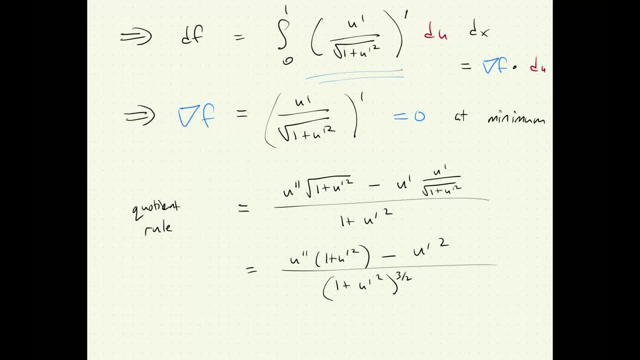 Okay, Yeah, Yeah, All right, Okay, Goodbye, Thank you, Bye, Bye, Bye, Bye, Bye. I'm just simplifying this a little bit. The second one: No, because this came from u prime times, u prime. 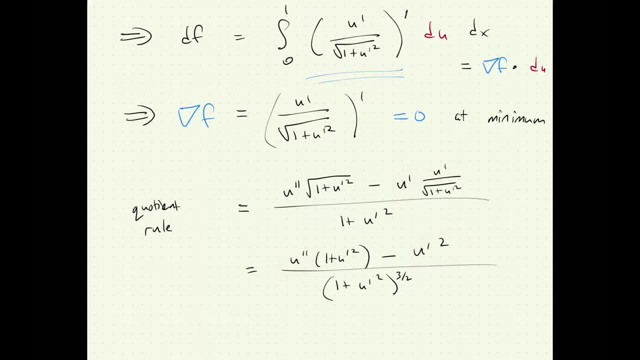 This one is u prime There. That came from this square root. I multiplied the top and the bottom by a square root of 1 plus u prime squared The second term. What's that This term? Are we talking about the right term or the left term? 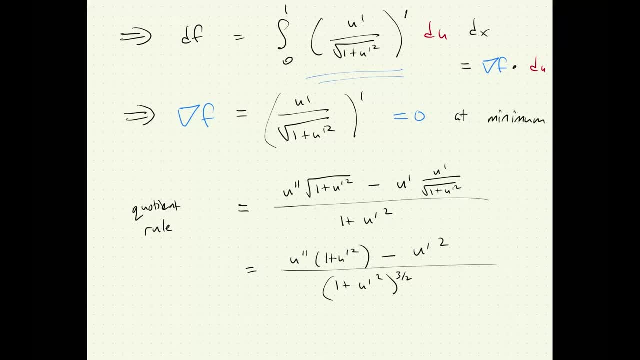 This one here. Sorry, You're saying this term is wrong. Did I make a mistake? Was this term correct? Oh, yes, Thank you. Oh, good, Good, Yeah, because that's going to screw things up, Okay. 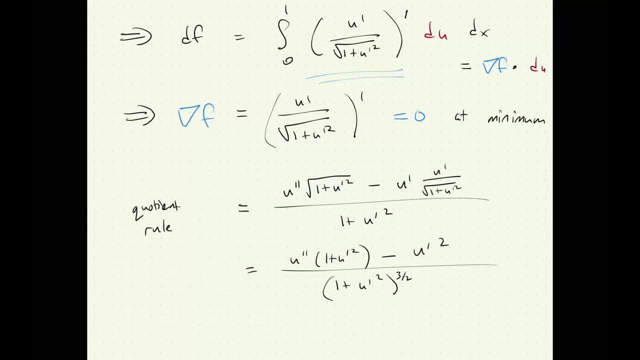 So yes, Okay, So good, Sorry. Yes, You're right. The top is not even that. It's u double primed Good, Okay, I knew something was supposed to cancel here. Good, It's actually u double primed times, u primed right. 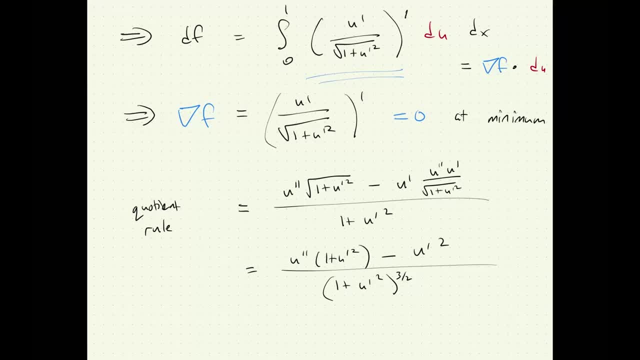 Okay, good, Because it's the derivative of u prime squared. It gives you 2 u double primed, U primed. The 2 canceled the derivative from the square root. Good, Good, I'm missing a u double primed error. 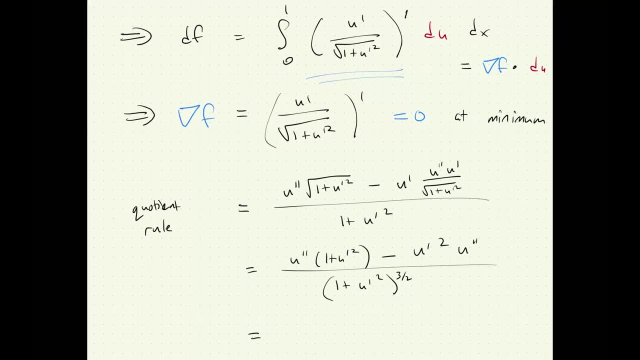 Ah good, I knew it was supposed to simplify. I was a little worried about that. So now this term cancels this term, And what you get is just u double primed over 1 plus u prime squared to the 3 halves. 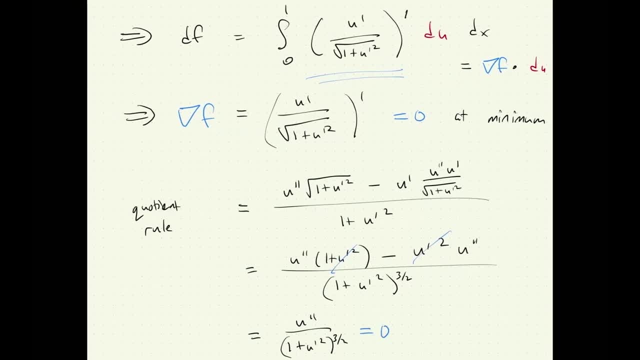 And this is supposed to equal 0, we said So. the only way it can be 0 is if u double primed is 0. So if u double primed equals 0, and that's a straight line, right. 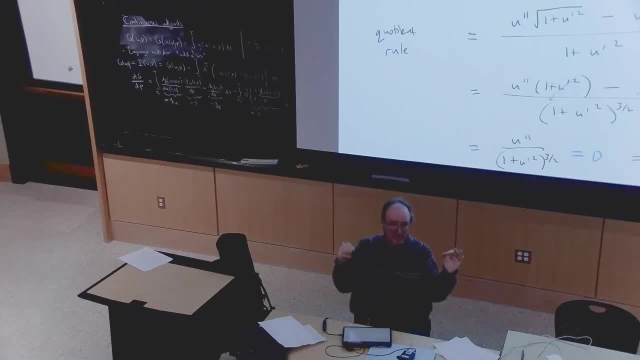 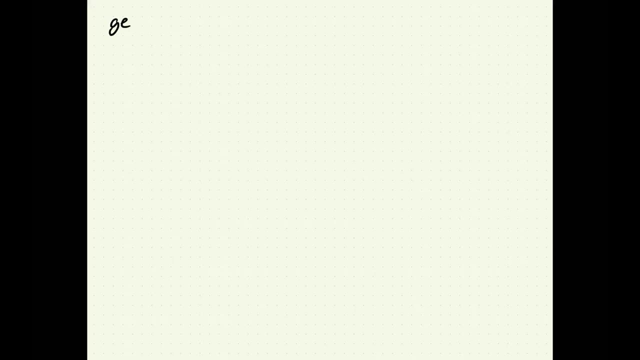 So what we've just derived is that the shortest distance between two points is a straight line. Of course you knew that right, But let's do a generalization, Okay. So let's say f Of u is an integral right from a to b right of some other function. 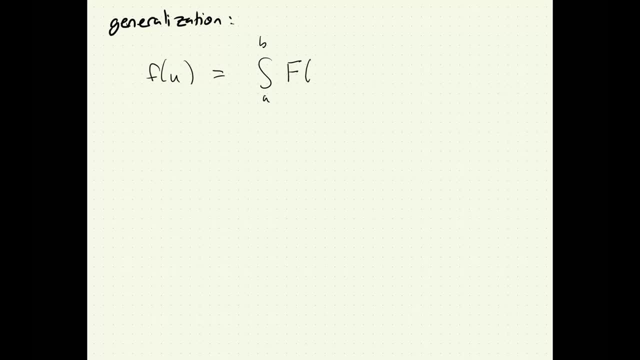 Let's call it capital F right of depends. It may depend on u, It may depend on u prime, It may depend on x right. This is a functional. And then what is df? So df is, you know again, f of u plus du minus f of u right. 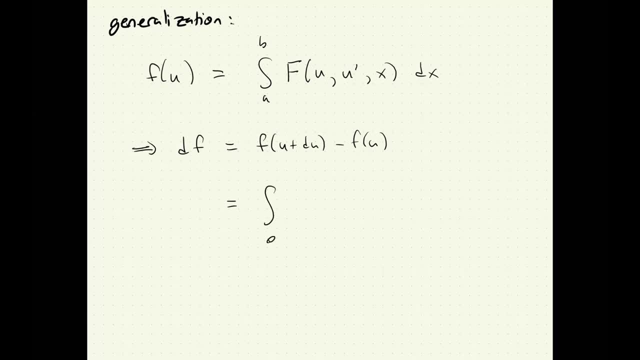 So now, what are we going to have? So there is going to be a term that looks like partial f, partial u. right, This is an ordinary 1801 partial derivative. I'm assuming u is a number. I guess it could be a vector. 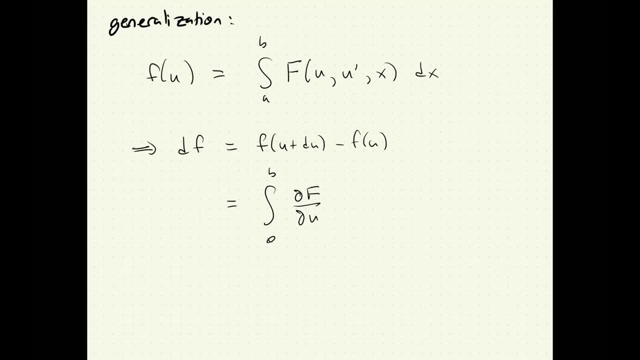 Something like that, But let's just keep it simple. Times du. There's also a term that looks like partial f, partial u primed times du. primed times dx. right, And this sometimes confuses people. It's like: how can I take the derivative with respect to u keeping u prime fixed? 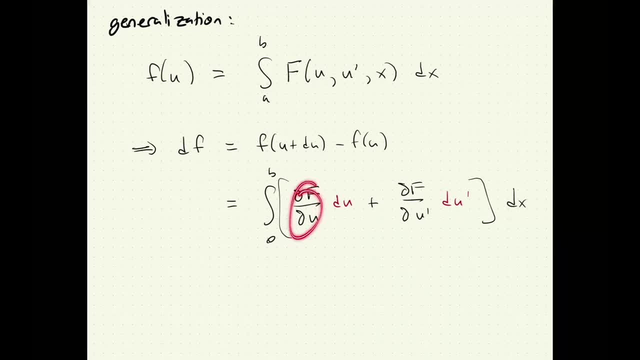 Because obviously u and u are related. It really means the derivative of f with respect to the first argument, right. This is the derivative of f with respect to the second argument, right. And then you plug in u and u prime afterwards, right. 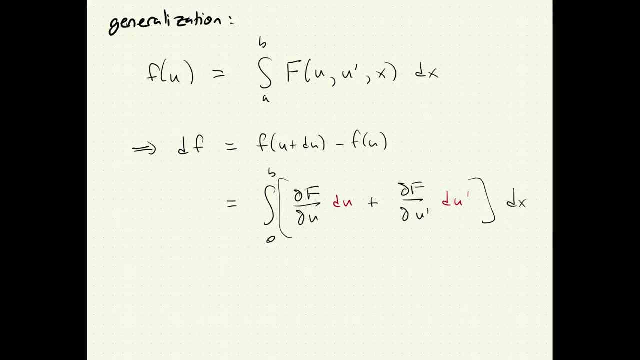 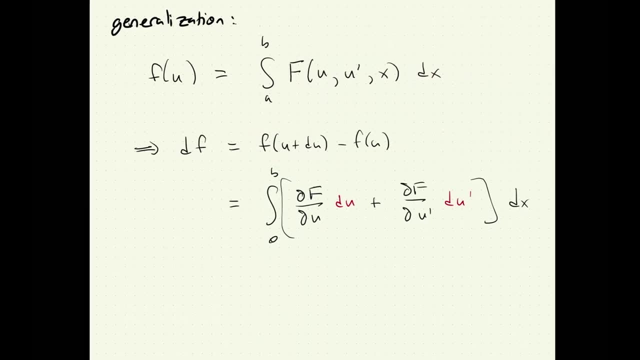 So it's just doing exactly the same and you're doing much like this in homework, right? I'm skipping a couple of steps here, but, right, This change. there's a change that comes from the first term, like we did on the first example, a sign of u. 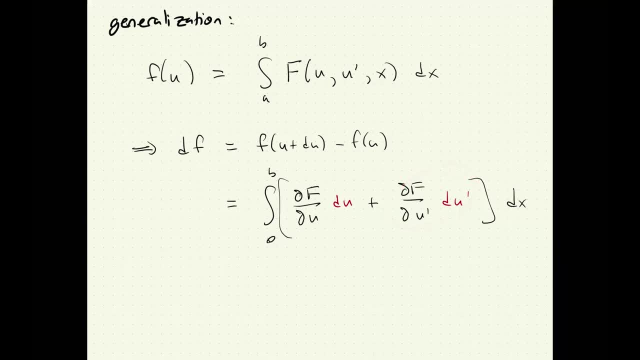 There's a change that comes from the second term, like in the second example, right And you have to add them up, But now you integrate by parts, right And on the du prime term, because we don't like having du primes. 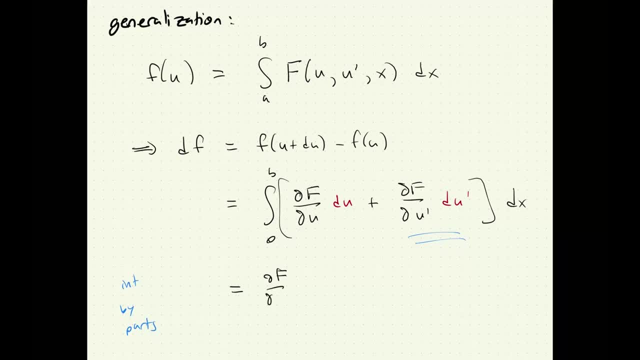 And so you get partial f, partial u, primed times du at a, b, And then we have a plus an integral a to b, And then there is a term, Okay, There's a term that looks like df du. 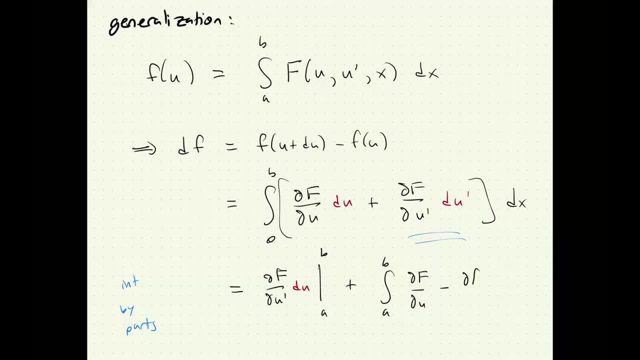 And there's another term that looks like with a minus sign: df, du, primed, primed. multiplying du times dx. Again, du is my small change, it's a du of x, right, I'm just suppressing all those. 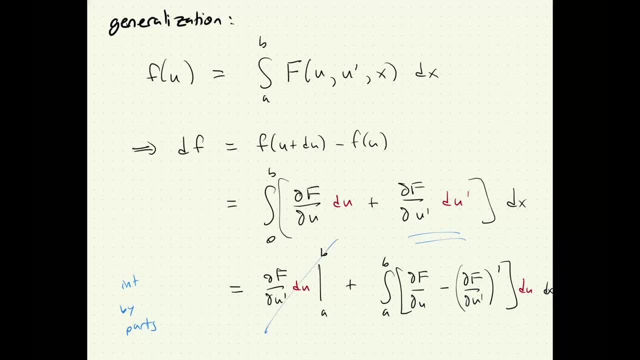 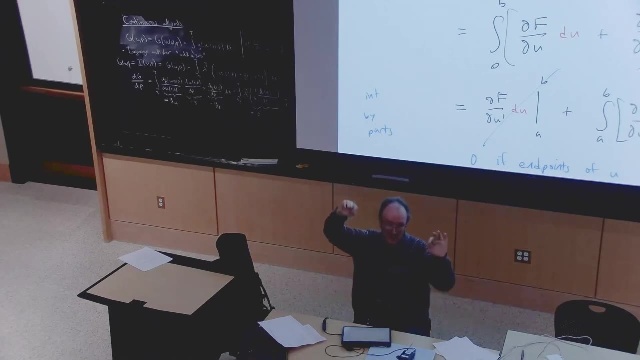 And this term we're going to set to zero if the end point, if the end points are fixed, of u are fixed. So if we keep u fixed at the end points, then we're going to only allow changes, du's that are arbitrary functions, but at the end points they have to be zero. 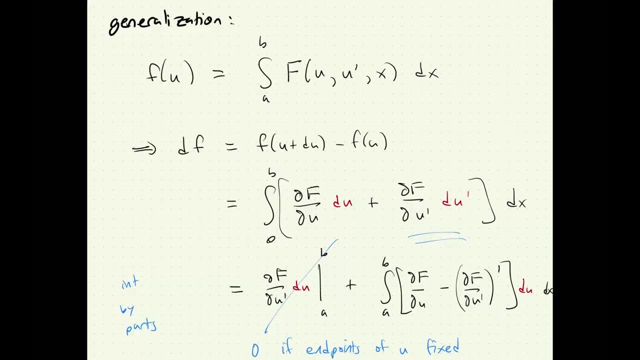 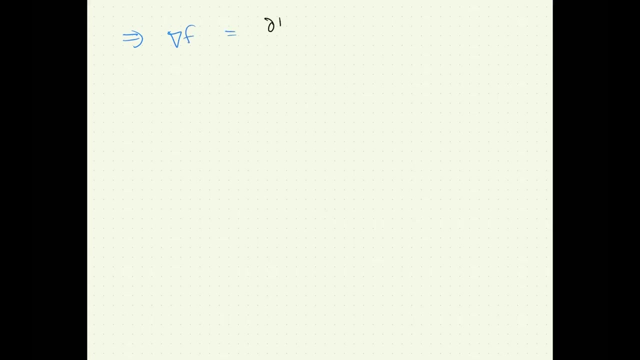 And so what you get is this term: here is the gradient. Okay, This is a grad f, All right, This is a dot product with du, and so I can write this out. So this is so. grad f is df du minus df du primed, primed. 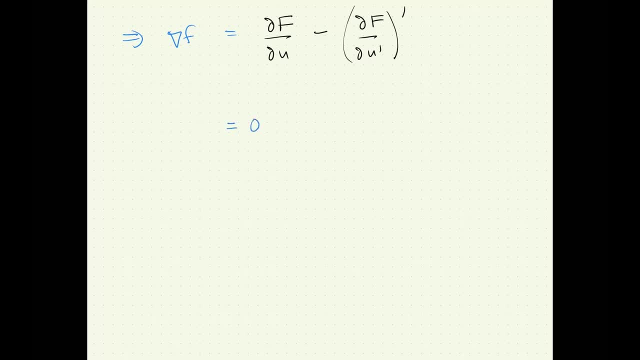 And we set this equal to zero at an extremum, at a minimum and maximum, And the result This is: we set this equal to zero. This is some differential equation. It's an equation in u right. It involves and it's actually a second order, right. 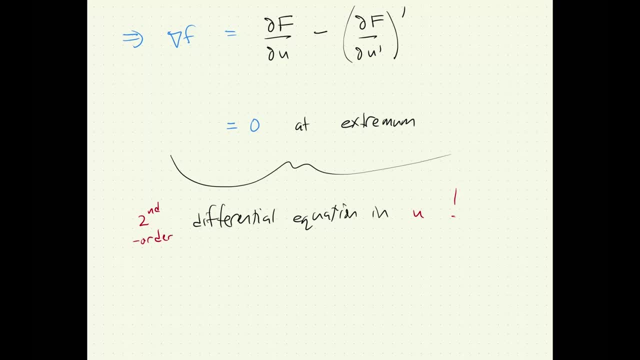 Because the way you started out with u and u primed in your f, but when I take this derivative here I'm going to get some u double primed terms. Does anyone know the name of this differential equation? Has anyone seen this before? 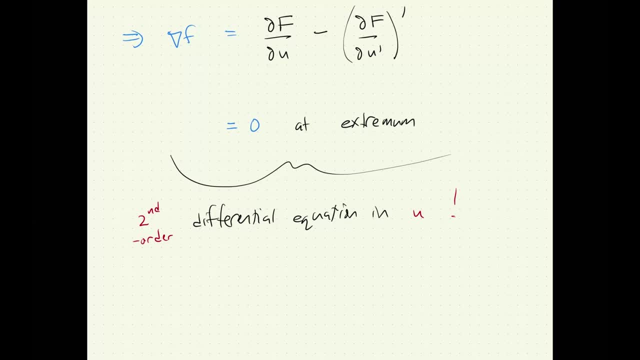 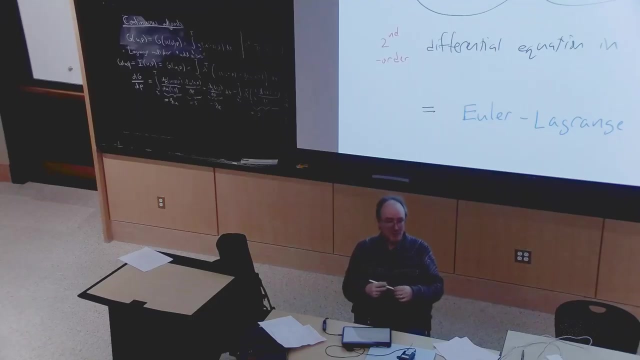 Euler-Lagrange equation. So this: these are exactly the Euler-Lagrange equations. Where did you see Euler-Lagrange equations before Optimal control, Optimal control. You also famously see them in advanced mechanics like 806 or 808.. 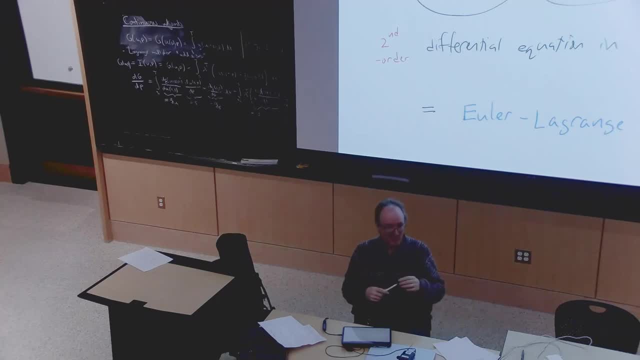 I don't know what the number is these days. Where this is, there's something called the least action principle And you can write down the equations of motion as minimizing some integral, And you get these Euler-Lagrange instead of Newton's laws. you get 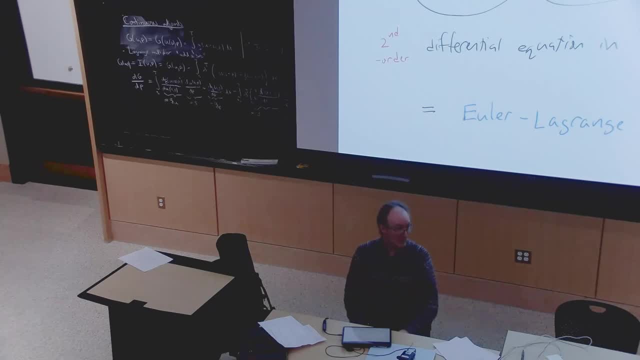 as a different way of getting Newton's laws. you get these Euler-Lagrange equations. They're really nice because they let you write down basically Newton's laws in like really weird coordinate systems pretty easily. Yeah, so there's a famous example of the Euler-Lagrange equation that everyone gives. 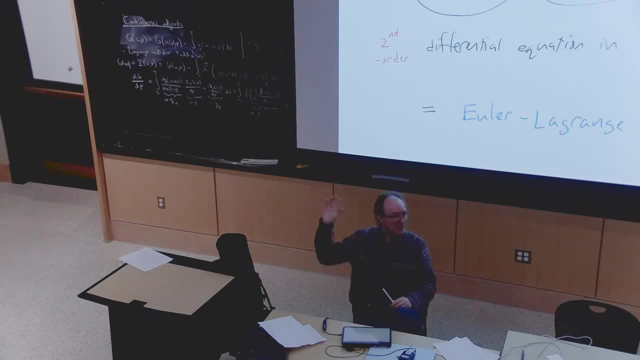 Which is called the Brachistochrone problem. Has anyone heard of the Brachistochrone problem? We have one person, a couple of people, right? So this is a famous problem from, I think, the 18th century. So suppose you have a mass falling down a slope. 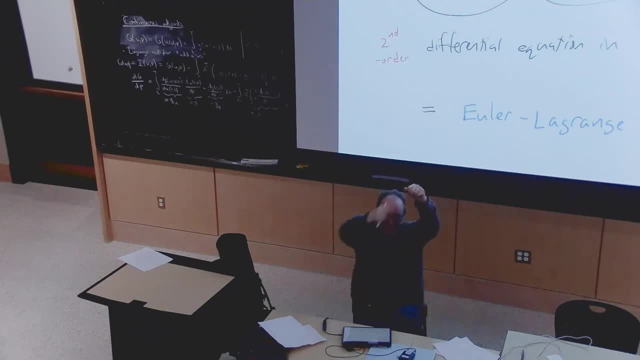 Just sliding down a curve. with gravity. It's going down this curve like a ramp, With no friction. Just slides down And you go. starting here, you're ending up here And the question is: what shape Should this ramp be to get down as quickly as possible? 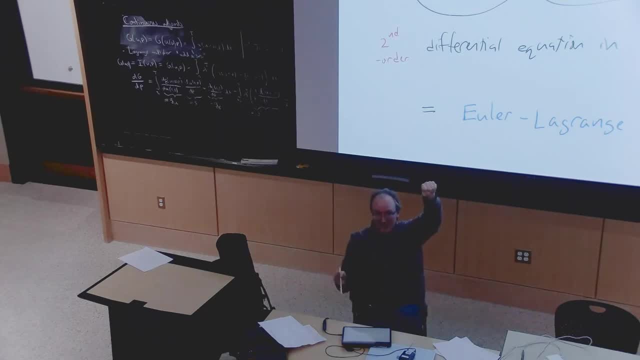 Should it be a straight ramp Or should it be like this? You can pretty easily see this shouldn't be like this, because then it'll start out going very, very slowly. A straight ramp, or it should go down very steeply and then flatten out. 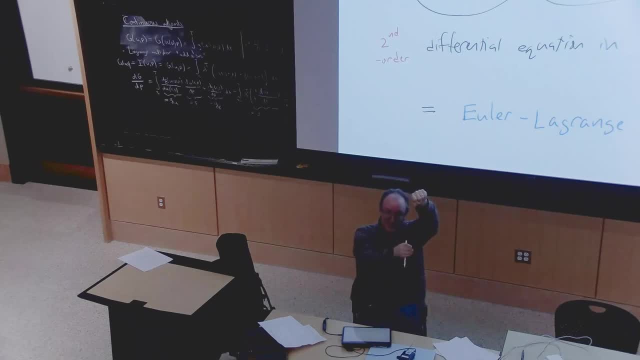 If it goes down very steeply it'll get going up, get a good head of speed pretty quickly, but then it has a longer distance. The straight line would be the shortest distance, but it's not the highest speed. So this is a famous problem called the Brichistochrone problem. 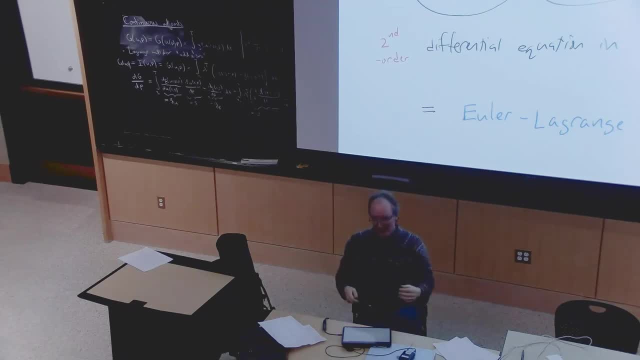 to find the curve of this ramp. that minimizes the time And it's exactly an integral. You can write down this And you write down a differential equation. You can solve it to get this curve. Unfortunately, the differential equation you get is rather nasty. 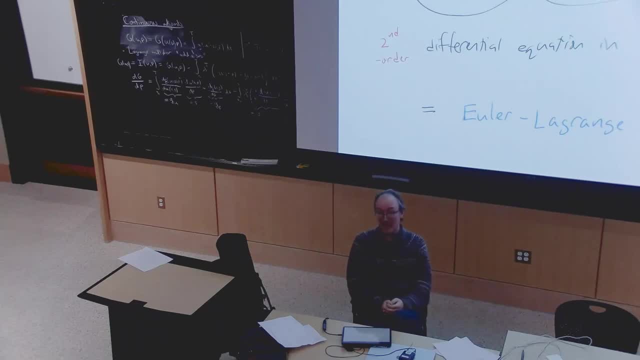 It is solvable in closed form, but it's nothing I would ever assign as a homework problem in 1803, for example. So it turns out, the minimum shape curve is called a cycloid. It's like a. It's the curve that if you have a wheel rolling, 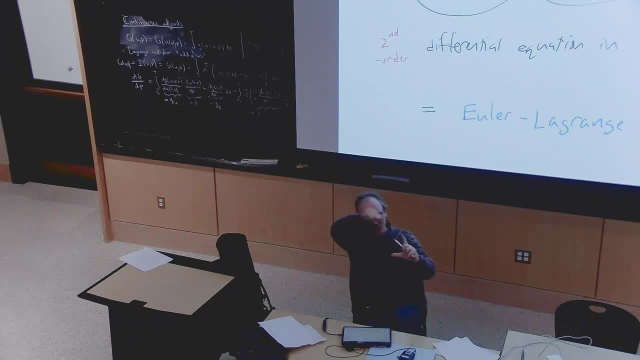 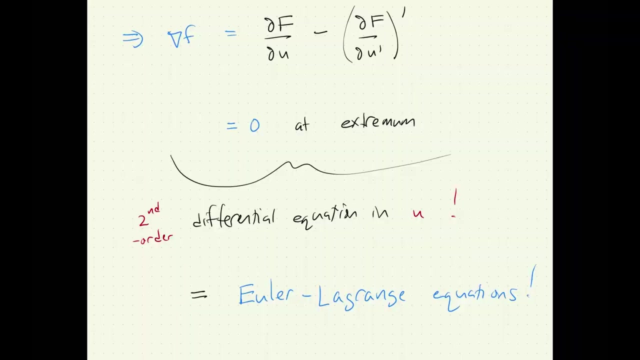 and you attach a pen to one spot on the wheel and, as it rolls, you mark out the curve that that wheel traces out. that's the shape that you get. So it's a famous. I'll even write that down. It's a Google example. 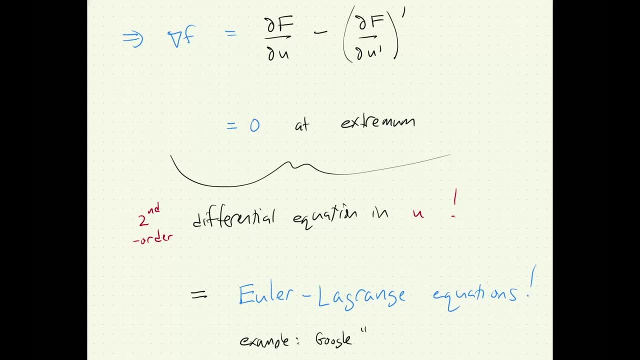 Google the Brichistochrone problem. Brichistochrone problem, That's one example. Another example would be: Google the principle of least action. That's how you get the Euler-Lagrange equations in mechanics. So great example, But it lets you turn these things around. 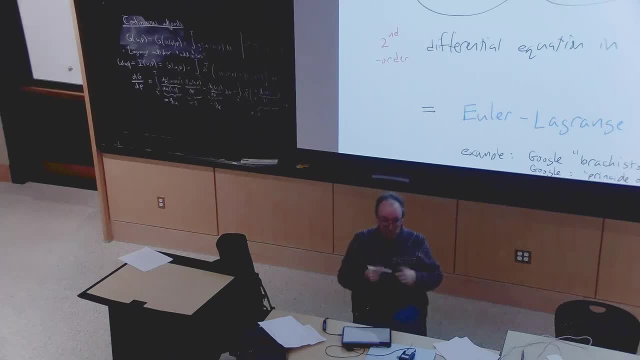 It lets you turn these things into different equations, But what you're really doing is just taking the gradient and setting it equal to zero, And it's just. you have to understand. okay, functions are a kind of vector. I can still talk about linear operators on functions.